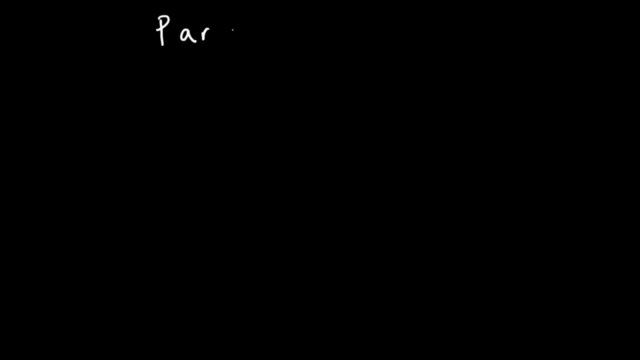 In this video we're going to focus on parallelograms. We're going to go over some properties associated with parallelograms and talk about how to solve some problems regarding it. So let's start with a picture. So let's say: this is A, B, C, D. So the first thing you need to 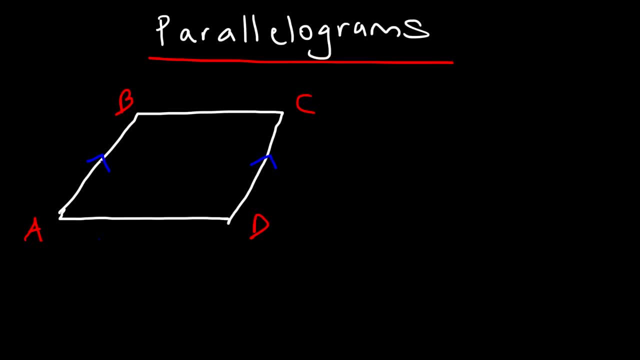 know is that opposite sides are parallel. So A- B is parallel to D C, And we could also say that B C is parallel to A D. Now, what else do we know regarding parallelograms? Well, for one thing, 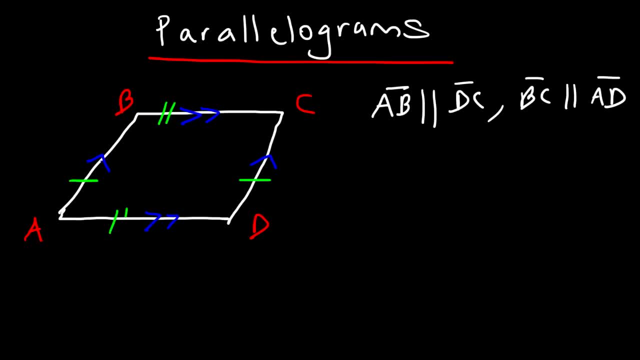 opposite sides are congruent. We could say A- B is congruent to D- C And also B- C is congruent to A- D. Now the next thing that we need to know is that opposite angles are congruent. So angle B: 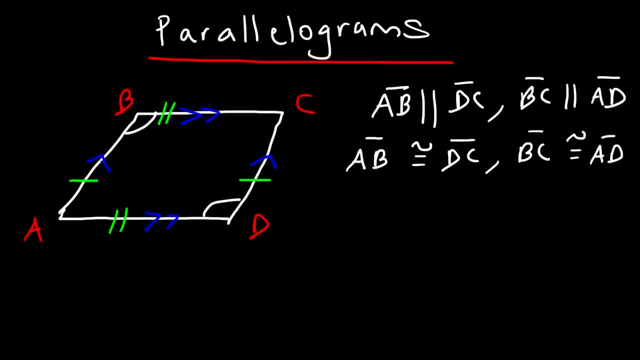 angle D are congruent to each other, and angle A and angle C are also congruent to each other. so let's say, if angle B is a hundred degrees, that means D is a hundred degrees. now what's the value of A and C? another rule you need to know is: 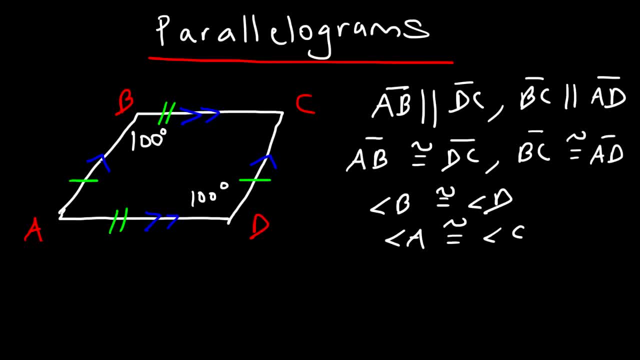 that consecutive angles are supplementary. so that means A and B have to add up to 180. B and C has to add up to 180. so A and C, they're equivalent to each other and they both must be 80. 100 plus 80 is 180 and so consecutive. 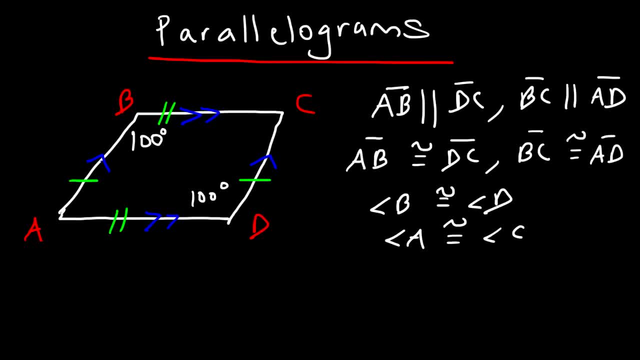 consecutive angles are supplementary, so that means A and B have to add up to 180. B and C has to add up to 180. so A and C, they're equivalent to each other and they both must be 80. a hundred plus 80 is 180, and so consecutive angles are: 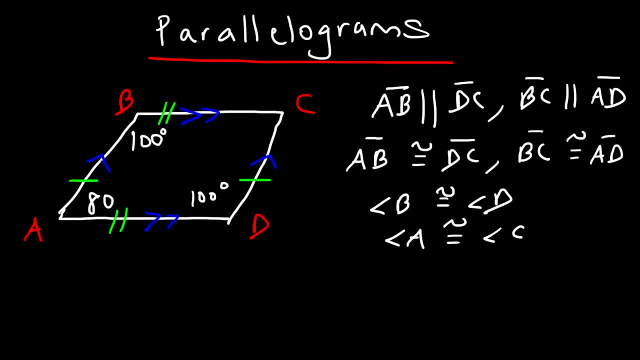 supplementary. now the next thing that you need to know is the diagonals. the diagonals bisect each other. so what does that mean? AC bisects BD and also BD bisects AC. so let's say: if AC is 20 units long, let's call this be. that means AE will be. 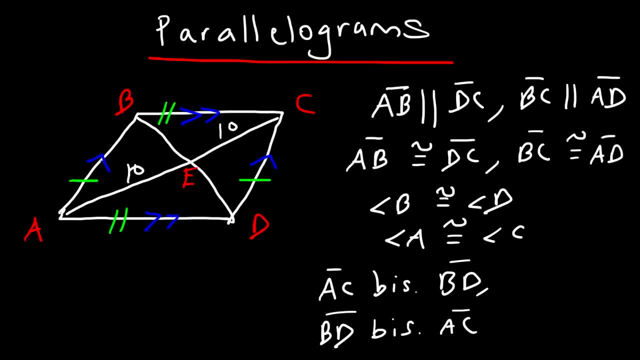 10 and EC will be 10. it's bisected into two congruent parts, so E is the midpoint of A and C. so let's say if BD was 12, that means be is 6 ed 6, and so it's important to understand that. 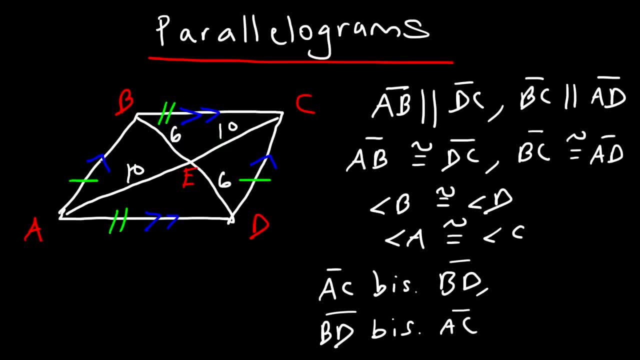 2, these two are congruent to each other, and so AE is one half of AC and AE is congruent to EC. so we can write that AE is congruent to EC and AE is basically one half of AC. so those are some other things that you want to keep in mind. 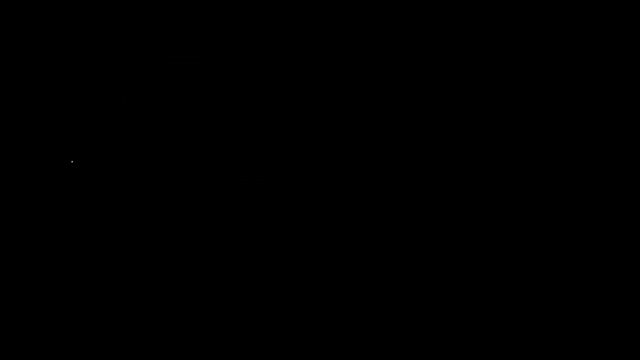 when dealing with parallelograms. now let's work on an example problem. so let's say: if we have parallelogram ABCD, now let's say that angle C is 9x minus 2 and angle D is 10x plus 30. with this information, calculate the measure of. 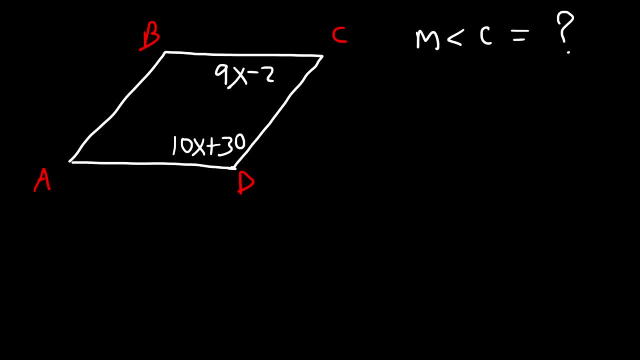 angle C. feel free to pause the video if you want to try it now. if you recall, consecutive angles are supplementary. so this means that angle C plus angle D must add to 180 degrees. so angle C is 9x minus 2, angle D is 10x. 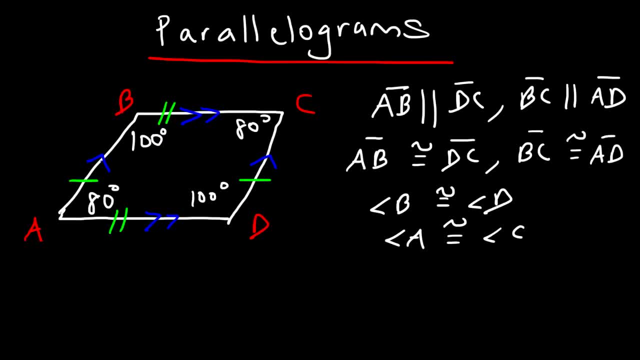 angles supplementary. now the next thing that you need to know is the diagonals. the diagonals bisect each other. so what does that mean? a C bisects BD and also BD bisects AC. so let's say: if AC is 20 units long, let's call this B. that means 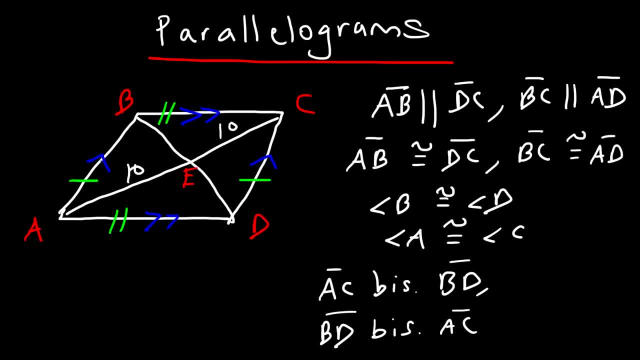 a, e will be 10 and EC will be 10. it's bisected into two congruent parts, so e is the midpoint of a and c. so let's say, if bd was 12, that means be is 6 ed 6, And so it's important to understand that these two are congruent to each other. 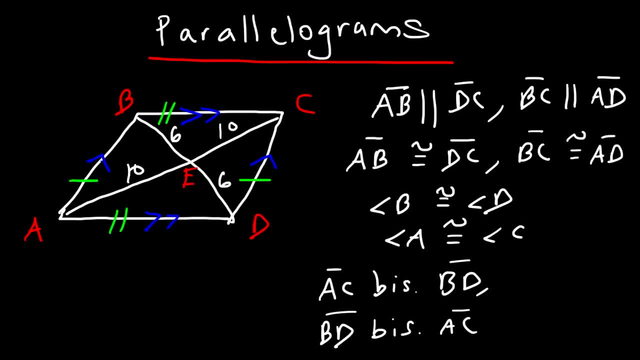 And so AE is one half of AC and AE is congruent to EC. So we can write that AE is congruent to EC And AE is basically one half of AC. So those are some other things that you want to keep in mind when dealing with parallelograms. 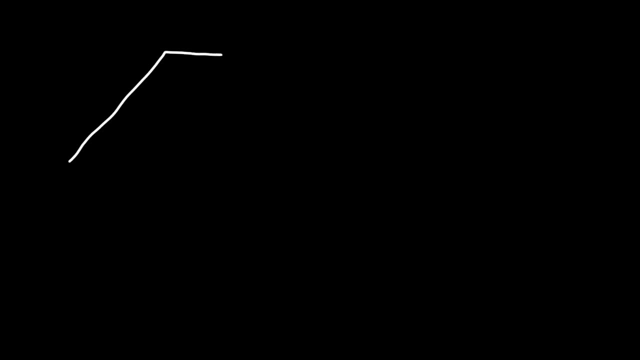 Now let's work on an example problem. So let's say, if we have parallelogram ABCD, Now let's say that angle C is 9x minus 2. And angle D is 10x plus 30. With this information, calculate the measure of angle C. 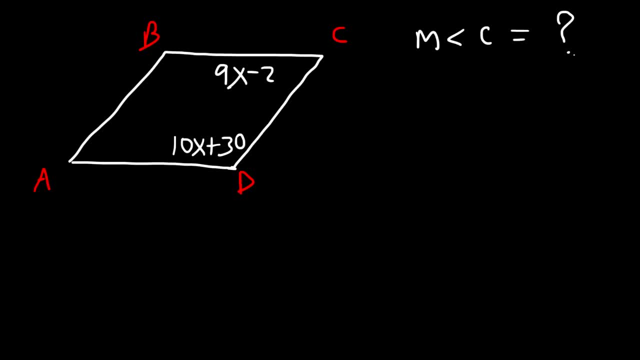 Feel free to pause the video if you want to try it Now. if you recall, we said that angle C is the measure of angle C. Now, if you recall, consecutive angles are supplementary. So this means that angle C plus angle D must add to 180 degrees. 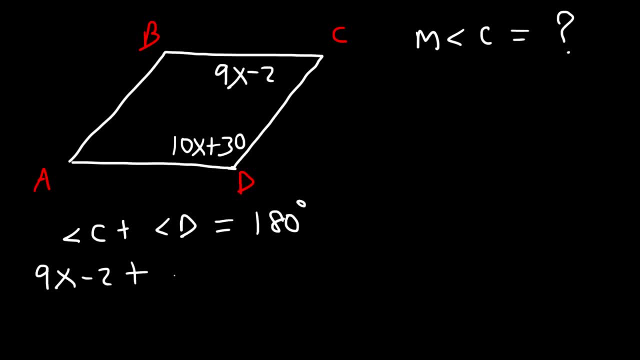 So angle C is 9x minus 2.. Angle D is 10x plus 30. So this has to add up to 180.. Now let's combine like terms: 9x plus 10x is 19x, Negative 2 plus. 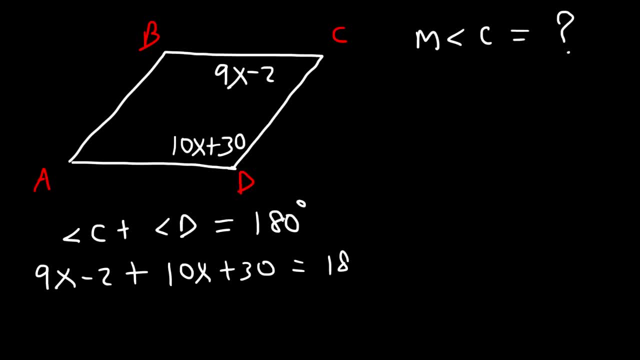 plus 30, so this has to add up to 180. now let's combine like terms: 9x plus 10x is 19x. negative 2 plus 30, that's 28. so now we need to subtract both sides by 28, so 180. 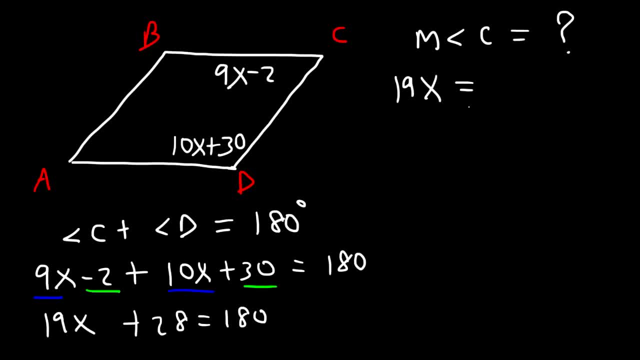 minus 28, that's 152. now let's divide both sides by 19. so 152 divided by 19 is 8. so now that we have the value of x, we can calculate the measure of angle C. so angle C is 9x minus 2. so let's plug in the x value that we have. so let's 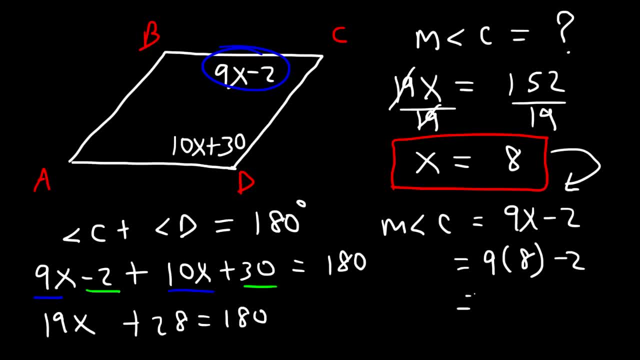 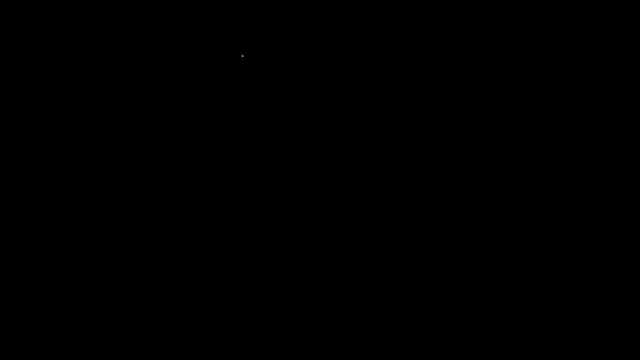 replace x with 8 and this will give us the answer. 9 times 8 is 72, and 72 minus 2 is 70, and so that's the measure of angle C, it's 70 degrees, and so that's it, for this problem is another example. so here we have a. 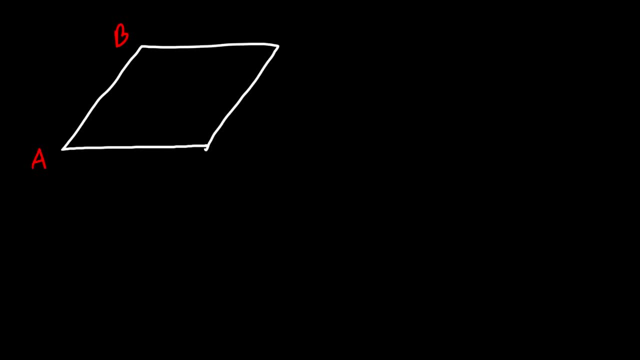 parallelogram. let's say once again: this is a, b, c and d. let's say that angle B is x squared plus 20 and angle D is seven X plus fifty. your task is to calculate the measure of angle C and D to架x vampire png. 0x50m lg d, drop thuentwenty's z2 and angle z2 h5. 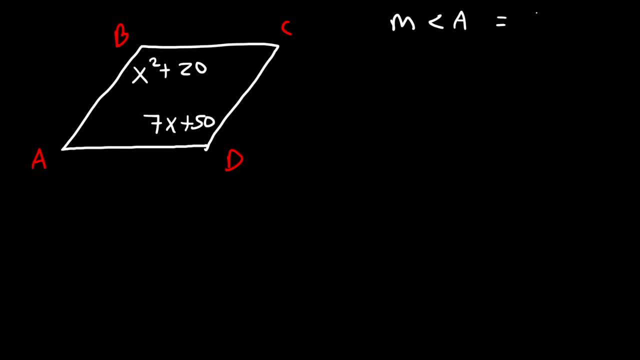 angle a. go ahead and do this. so one rule that you need to remember for parallelograms is that opposite angles are congruent. so this means that angle B is equal to angle D. so B is x squared plus 20 and D is 7x plus 50. so let's go. 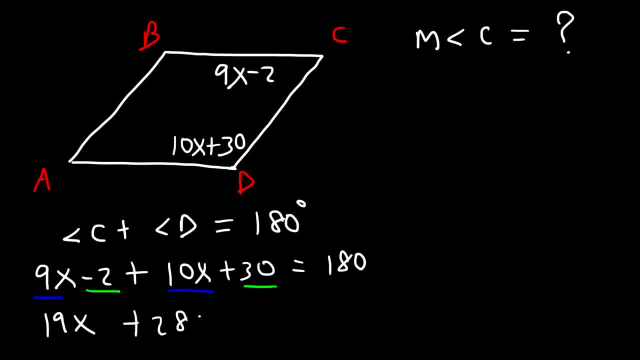 Negative: 2 plus 30,, that's 28.. So now we need to subtract both sides by 28.. So 180 minus 28, that's 152.. Now let's divide both sides by 19.. So 152 divided by 19 is 8.. 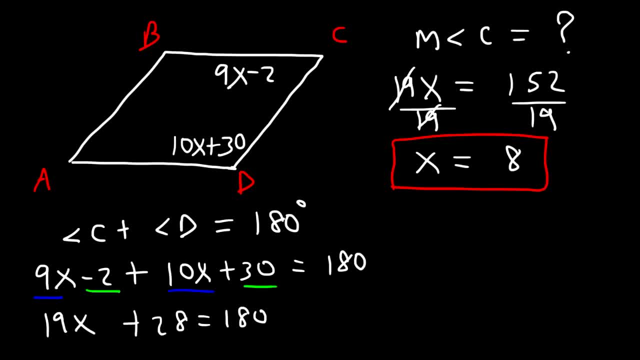 So now that we have the value of x, we can calculate the measure of angle C. So angle C is 9x minus 2.. So let's plug in the x value that we have. So let's replace x with 8,. 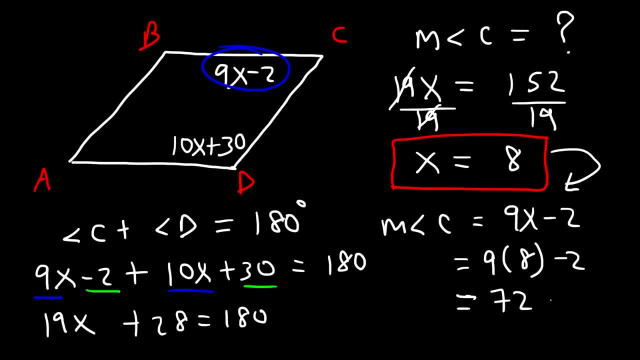 and this will give us the answer: 9 times 8 is 72.. And 72 minus 2 is 70.. And so that's the measure of angle C: It's 70 degrees, And so that's it for this problem. 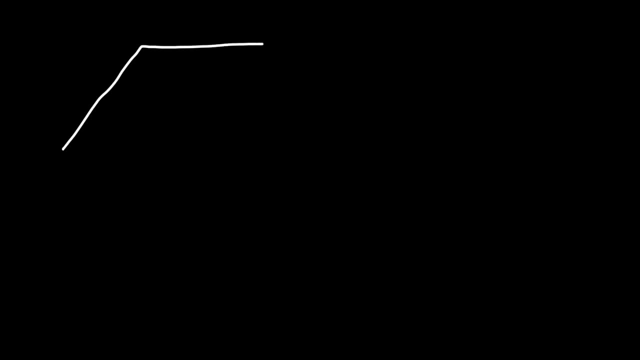 Here's another example. So here we have a parallelogram And let's say once again: this is A, B, C and D. Let's say that angle B is x squared plus 20.. And angle D is 7x plus 50.. 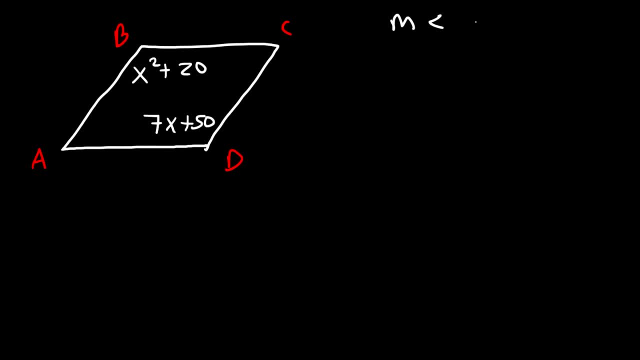 Your task is to calculate the measure of angle A And go ahead and do this. So one rule that you need to remember for parallelograms is that opposite angles are congruent. So this means that angle B is equal to angle D, So B is x squared plus 20.. 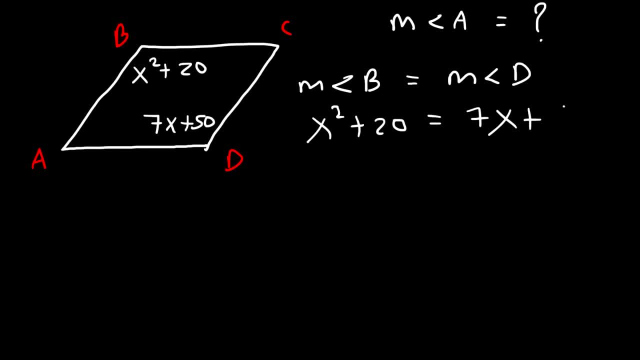 And D is 7x plus 50.. So let's go ahead and calculate the value of x. So how should we do this? The best thing is to take everything on the right side and move it to the left side, So it's going to be x squared minus 7x plus 20 minus 50.. 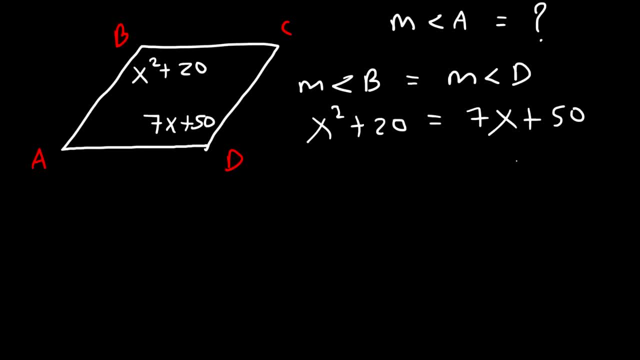 ahead and calculate the value of x. so how should we do this? the best thing is to take everything on the right side and move it to the left side, so it's going to be x squared minus 7x, plus 20 minus 50. now, 20 minus 50 is: 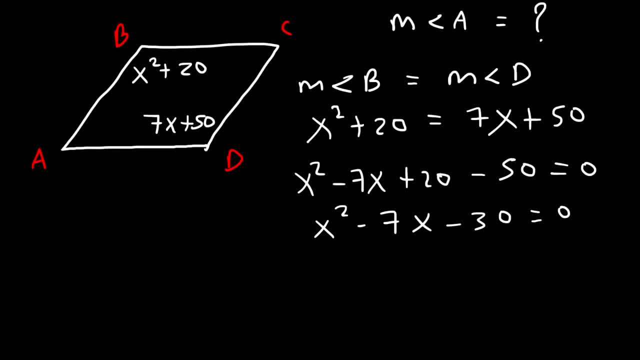 negative 30. so this is what we now have. so what two numbers we need to factor this quadratic equation? by the way, what two numbers multiply to negative 30 but add to the middle coefficient negative 7? we need to find two numbers that multiply to negative 30 and add to negative. 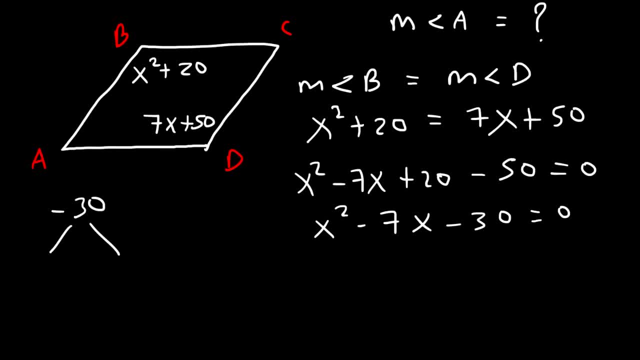 7. this will help us to factor this trinomial. so we have 2 and 15, 3 and 10, 5 and 6. notice that 3 and 10 differs by 7 and to make it negative, 30, one of them. 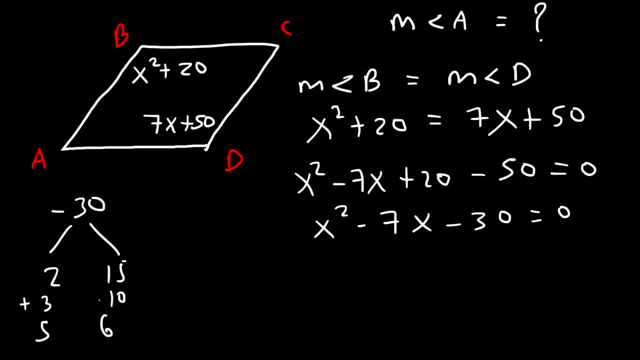 have to be negative. so it makes sense if we make it positive 3 and negative 10 3 times negative 10 is negative 30, but 3 plus negative 10 adds up to negative 7, so to factor it's going to be x plus 3 times x minus 10. now what we need to do: 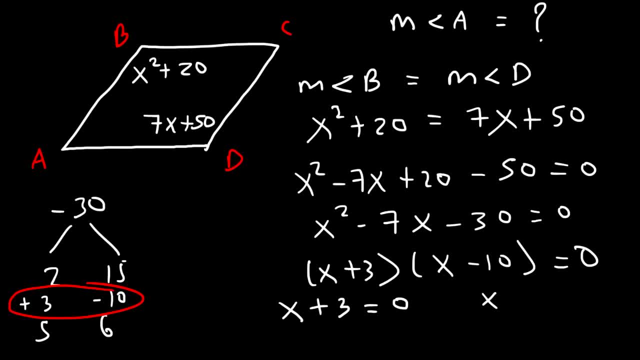 is set both factors equal to 0, and so we can see that x will equal 3- I mean negative 3. if we subtract both sides by 3, and if we add 10 to both sides, x will equal positive 10. so it looks like we may have two possible. 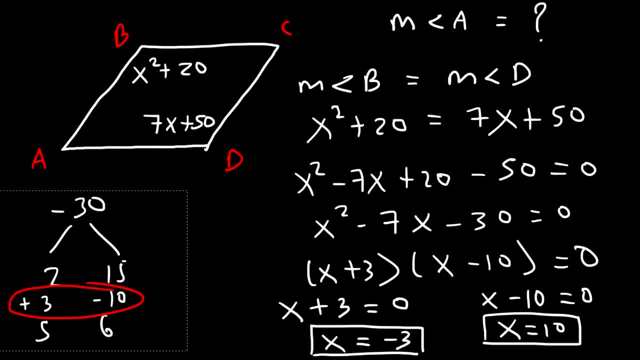 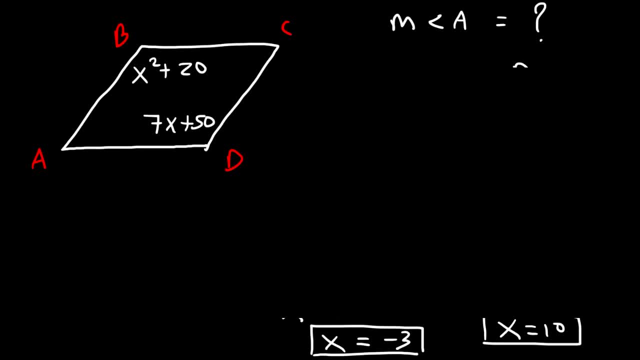 answers. if we plug in negative 3, both angle B and angle D will be the same and they will both have a positive measure. so, for example, the measure of angle B is going to be x squared plus 20, and so that's negative 3 squared plus 20. 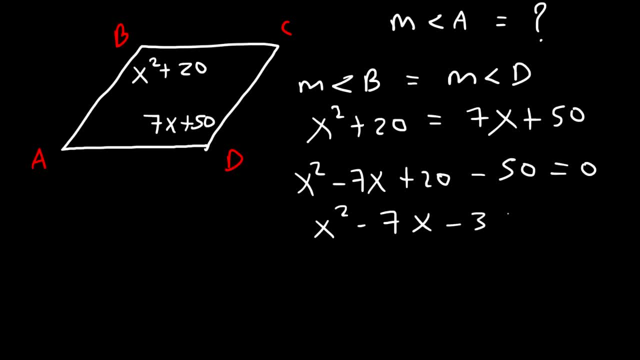 Now, 20 minus 50 is negative 30. So this is what we want to do. This is what we now have. So what two numbers We need to factor this quadratic equation, by the way, What two numbers multiply to negative 30? 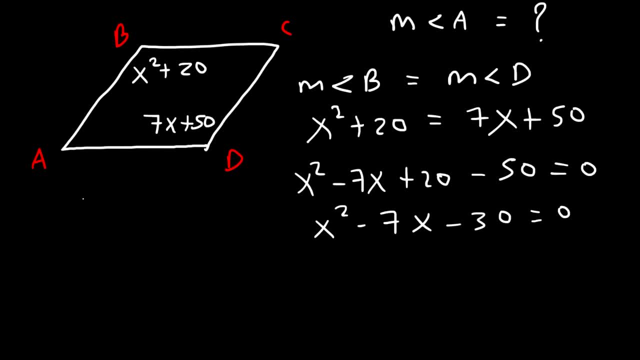 but add to the middle coefficient negative 7? We need to find two numbers that multiply to negative 30 and add to negative 7.. This will help us to factor this trinomial. So we have 2 and 15,, 3 and 10,, 5 and 6.. 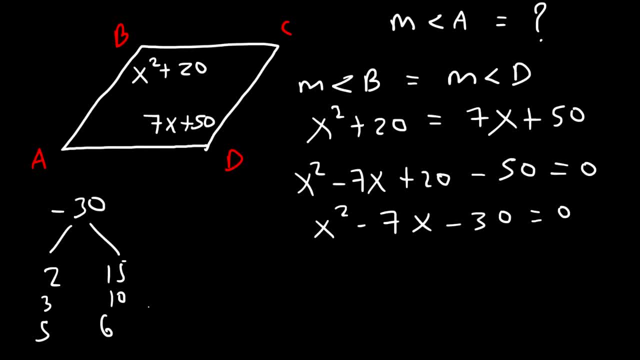 Notice that 3 and 10 differs by 7.. And to make it negative 30,, one of them has to be negative. So it makes sense if we make it positive 3 and negative 10.. 3 times negative 10 is negative 30,. 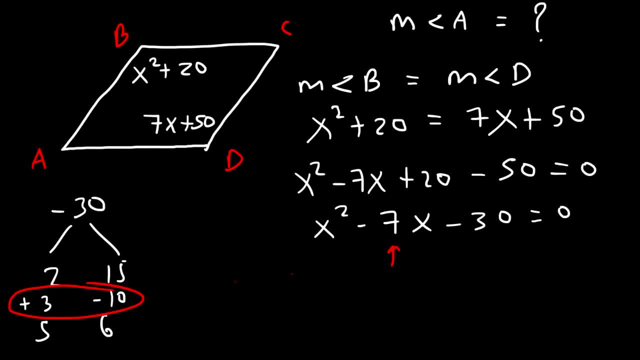 but 3 plus negative 10 adds up to negative 7.. So to factor it, it's going to be x plus 3 times x minus 10.. Now what we need to do is set both factors equal to 0. And so we can see that x will equal 3, I mean negative 3,. 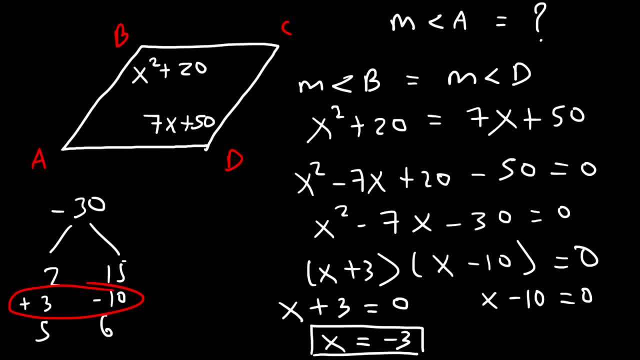 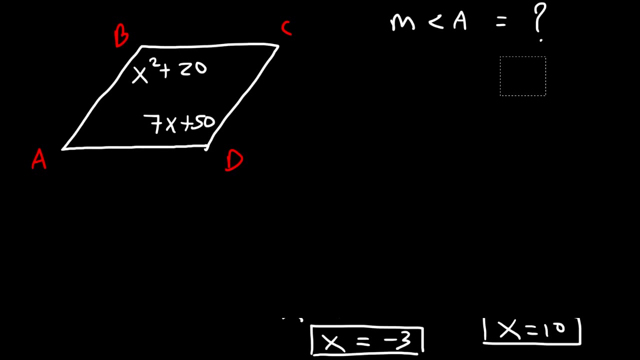 if we subtract both sides by 3. And if we add 10 to both sides, x will equal positive 10.. So it looks like we may have two possible answers. If we plug in negative 3,, both angles are going to be equal to 0. 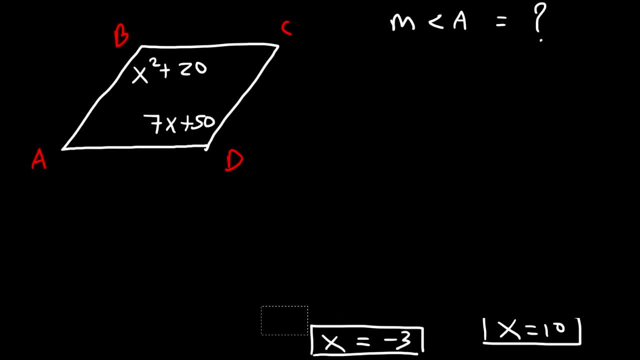 So angle B and angle D will be the same, and they will both have a positive measure. So, for example, the measure of angle B is going to be x squared plus 20.. And so that's negative 3 squared plus 20, which is 9 plus 20.. 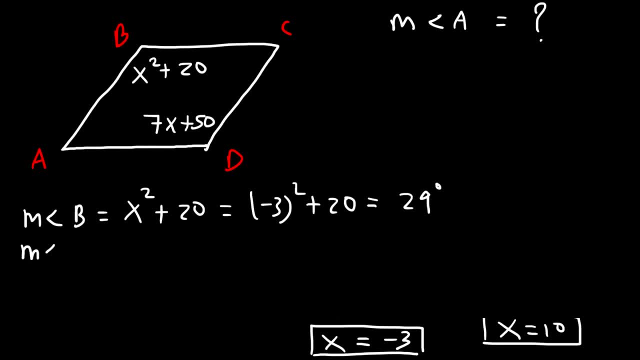 So that's 29 degrees, And angle D will have the same value. It's going to be 7 times negative 3 plus 50.. 7 times negative 3 is negative 21.. Plus 50, that's 29 degrees. 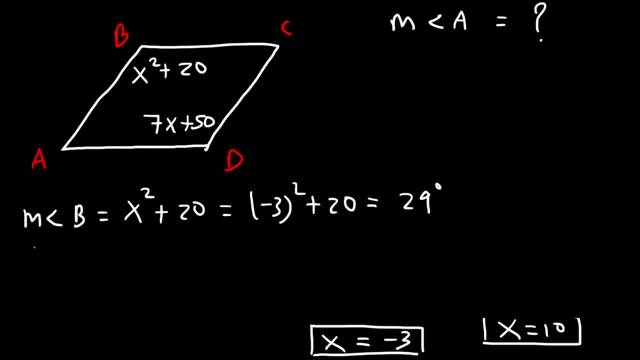 which is 9 plus 20, so that's 29 degrees, and angle D will have the same value. it's going to be 7 times negative, 3 plus 50. 7 times negative 3 is negative 21 plus 50, that's 29 degrees. so one possible answer for angle B is: 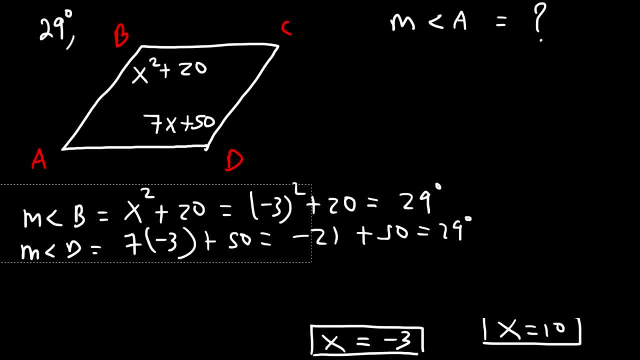 29, let's see what the other possible answer is going to be. so let's say: if X is 10, so angle B is going to be 10 squared plus 20. 10 squared is 100, 100 plus 20, that's 120 degrees. and if we check, 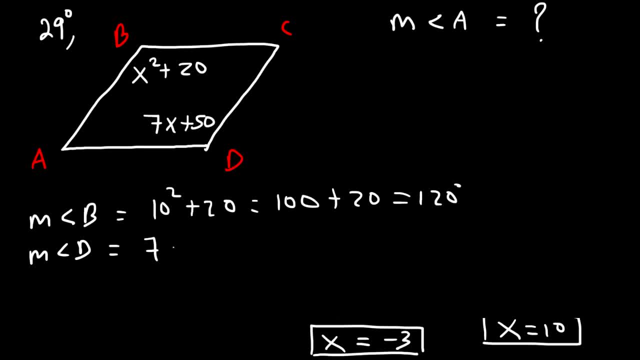 it by calculating angle D, it's going to be 7 times 10 plus 50, so that's 70 plus 50, which is also 120. so angle B can be 29 or 120 degrees. so now we can find the possible answers for angle a. keep in mind that a and B are supplementary, so the measure 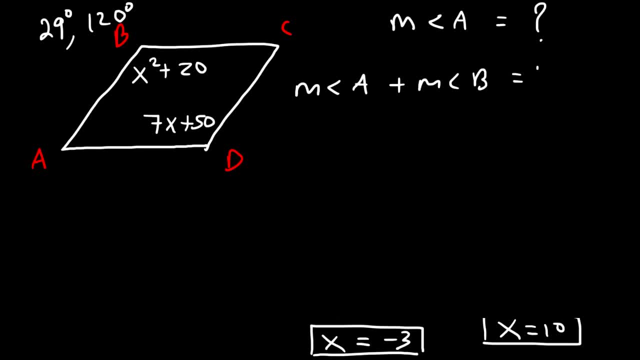 of a plus the measure of B has to add up to an 80. so let's calculate a. if B is 29, so that's going to be 180 minus 29. so one possible answer for angle a is 151 degrees. now the other possible answer is 180 minus 120, so it could be 60. so there's. 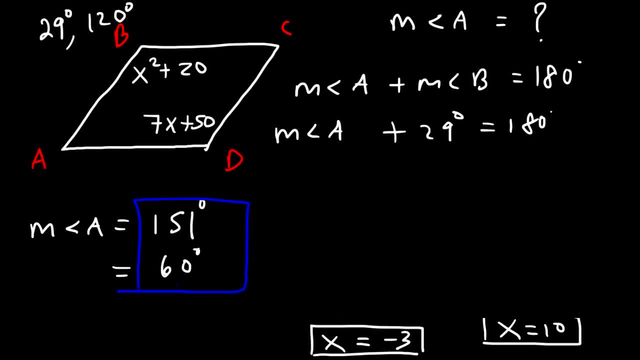 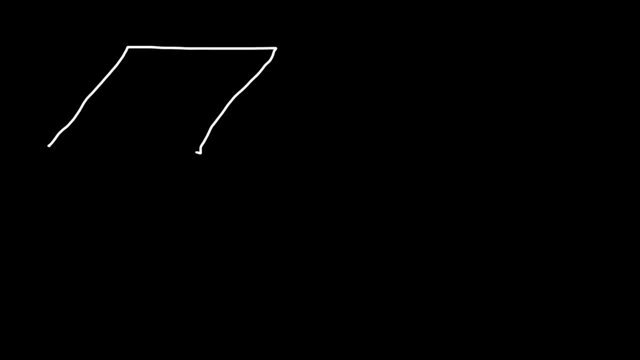 two possible answers for this angle: it could be 60 degrees or 151. now let's work out another example. so this is going to be a, B, C and D, as usual, and this time we're going to have some diagonals, and let's call this point E. so 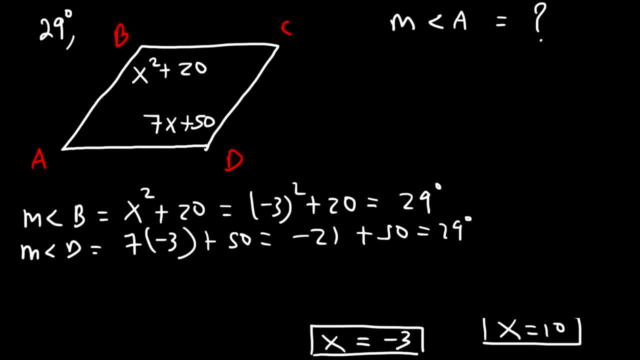 So one possible answer for angle B is 29.. Let's see what the other possible answer is going to be. So let's say if x is 10.. So angle B is going to be 10 squared plus 20.. 10 squared is 100.. 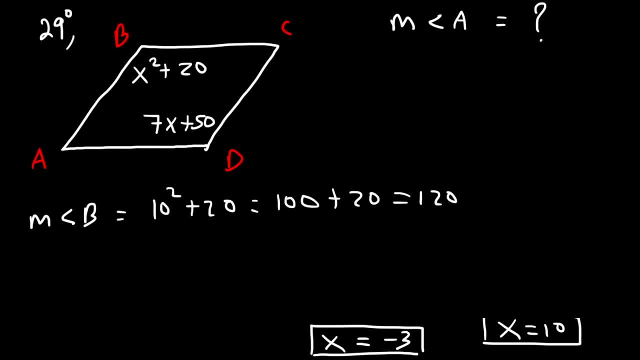 100 plus 20,, that's 120 degrees, And if we check it by calculating angle D, it's going to be 7 times 10 plus 50.. So that's 70 plus 50, which is also 120.. 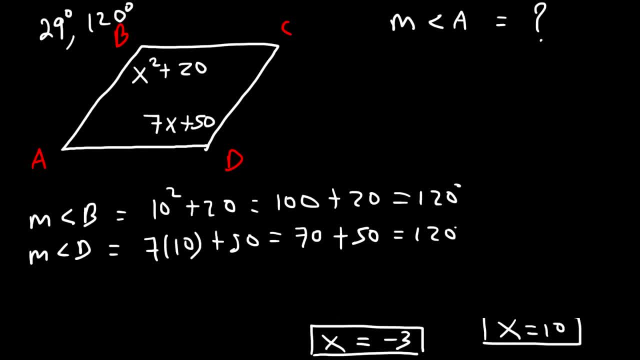 So angle B can be 29 or 120 degrees. So now we can find the possible answers for angle A. Keep in mind that A and B are supplementary. So the measure of A is a. So the measure of A is a. So the measure of A is a. 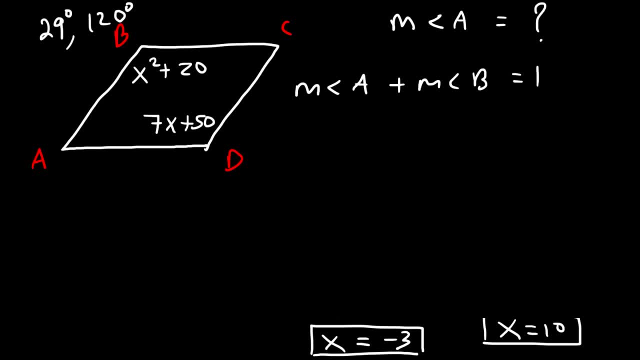 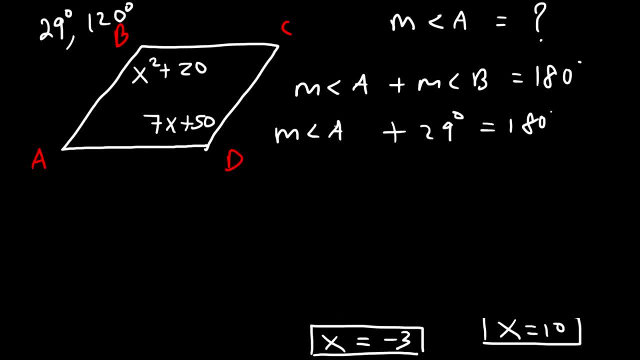 So that's going to be 180 minus 29.. So one possible answer for angle A is 151 degrees. Now the other possible answer is 180 minus 120.. So it could be 60.. So there's two possible answers for this angle: It could be 60 degrees or 151.. Now let's work out another example. 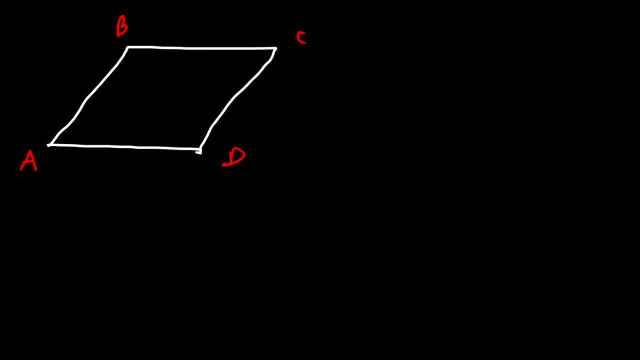 So this is going to be A, B, C and D, as usual, And this time we're going to have some diagonal Diagonals And let's call this point E. So A E in this problem is going to be 4x. 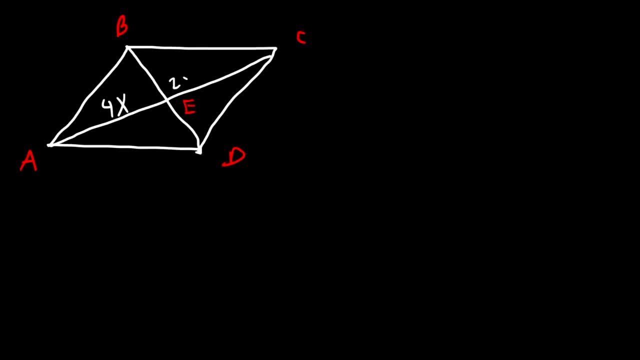 And E C, we're going to say it's 2x squared minus x minus 3.. So, knowing this, what is the measure? What is the length of A C? Go ahead and work on this problem. Now, if you recall, the diagonals bisect each other. 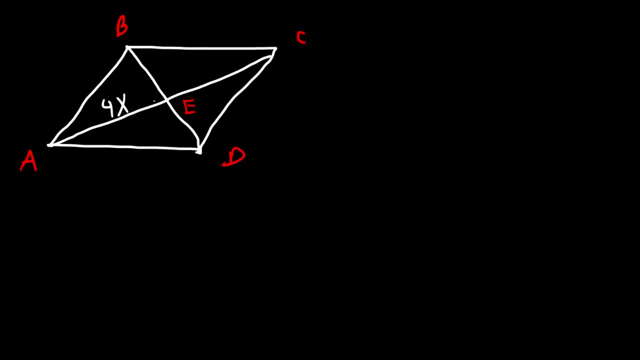 a, E, and this problem is going to be 4x and EC. we're going to say it's 2x squared minus x, minus 3. so, knowing this, what is the measure? what is the length of a, C, g, g, g, g, g? ahead and work on this problem. Now, if you recall, the diagonals bisect each other. So 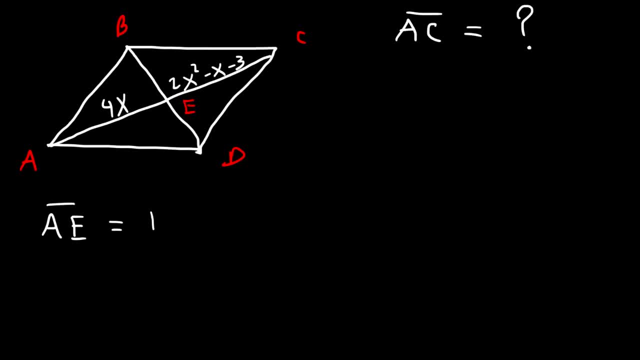 what that means is that AE is equal in length to EC. These two sides are equivalent to each other. So therefore we could set AE, which is 4x, equal to EC, which is 2x squared minus x minus 3.. So we have another quadratic equation. So let's begin by subtracting both sides by 4x. 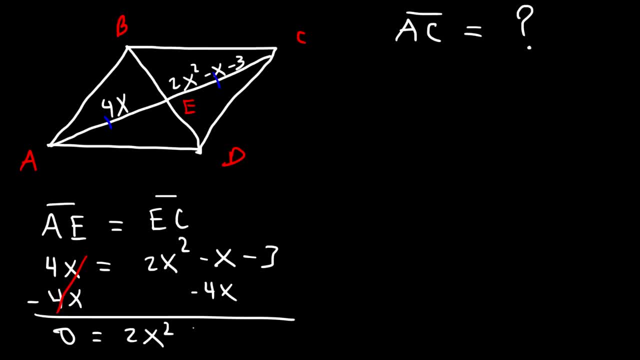 So this is going to be: 0 is equal to 2x squared Negative 1x minus 4x is negative 5x, And so we have this expression. So how can we factor 2x squared minus 5x minus 3?? 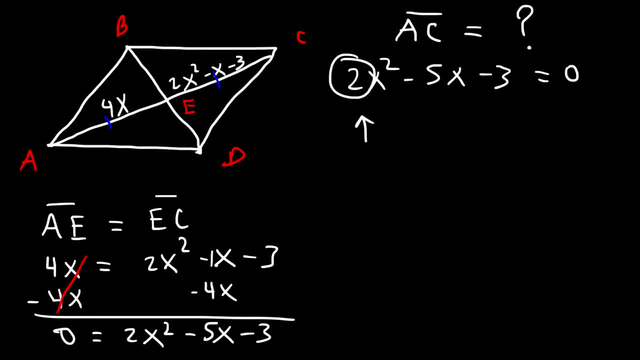 So notice that we have a trinomial where the leading coefficient is not 1.. So what do we need to do in this case? The first thing you need to do is you need to multiply the leading coefficient by the constant term. So 2 times negative, 3 is negative 6.. Next, you need to find two numbers that multiply to: 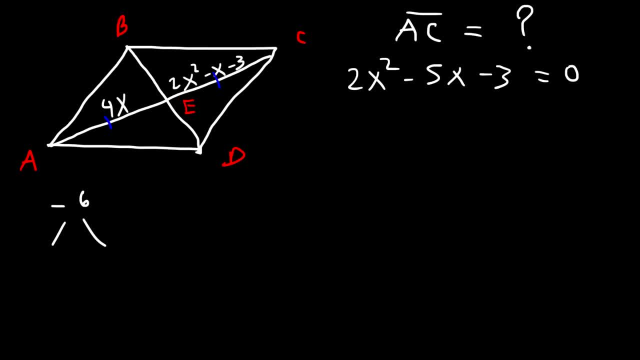 negative 6, but add to the middle coefficient negative 5.. This is going to be negative 6 and positive 1.. Negative 6 plus 1 adds to the middle coefficient negative 5.. So we have a trinomial that's up to negative 5.. Next, replace the middle term with these two. 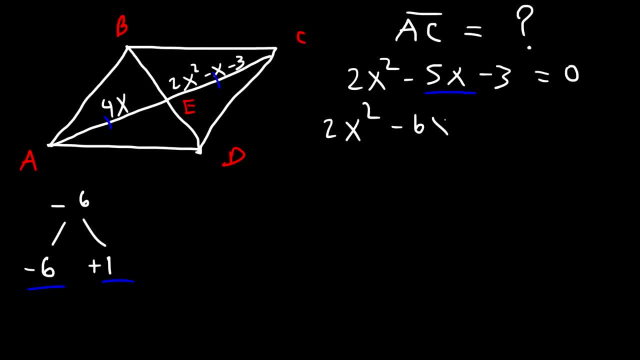 So we're going to replace negative 5x with negative 6x plus 1x, because they add up to negative 5x After that factor by grouping. So in the first two terms, take out the GCF, the greatest common factor. In this case it's going to be 2x, 2x squared divided by 2x. 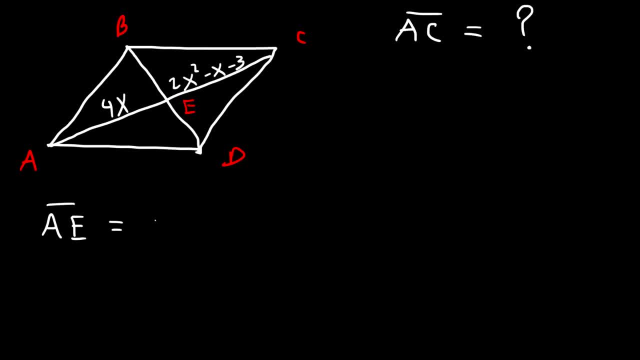 So what that means is that A E is equal in length to E C. These two sides are equivalent to each other, So therefore we could set A E, which is 4x equal to E C, which is 2x squared minus x minus 3.. 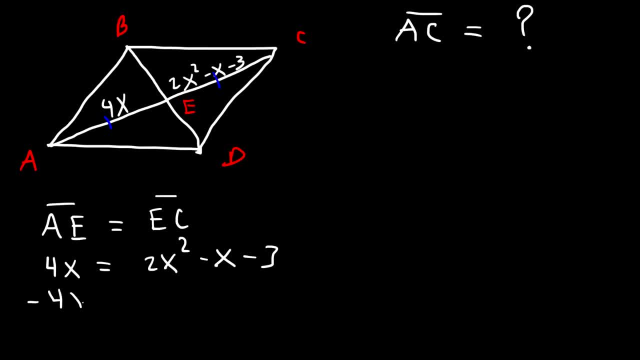 So we have another quadratic equation. So let's begin by subtracting both sides by 4x. So this is going to be: 0 is equal to 2x squared Negative 1x minus 4x is negative 5x. 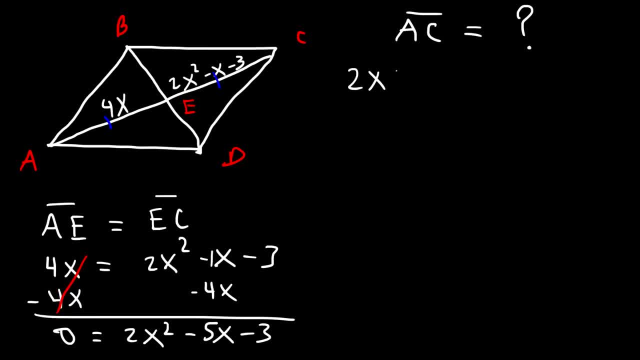 And so we have this expression. So how can we factor 2x squared minus 5x minus 3?? So notice that we have a trinomial where the leading coefficient is not 1.. So what do we need to do in this case? 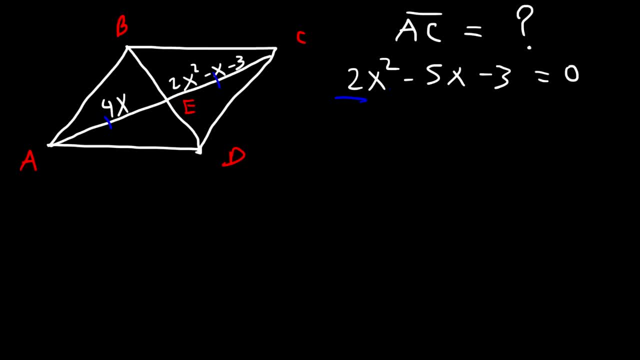 The first thing you need to do is you need to multiply the leading coefficient by the constant term. So 2 times negative 3 is negative 6.. Next, you need to find two numbers that multiply to negative 6 but add to the middle coefficient negative 5.. 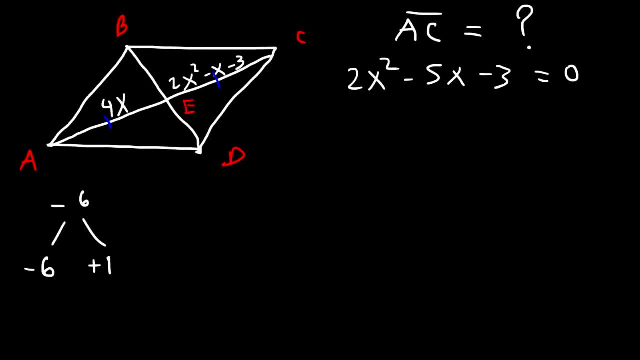 This is going to be negative 6 and positive 1.. Negative 6 plus 1 adds up to negative 5.. Next, replace the middle term with these two. So we're going to replace negative 5x with negative 6x plus 1x, because they add up to negative 5x. 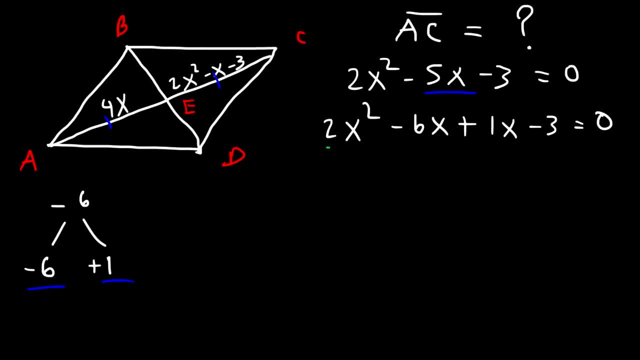 After that factor by grouping. So in the first two terms, take out the GCF, the greatest common factor. In this case it's going to be 2x. 2x squared divided by 2x is x Negative. 6x divided by 2x is negative 3.. 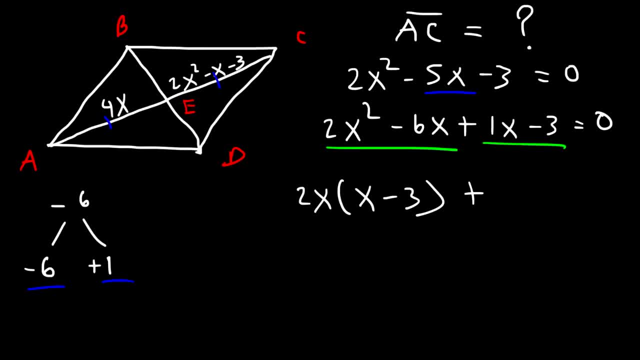 Now, in the last two terms, we're going to have to multiply the leading coefficient by the constant term. So in the last two terms, factor out the GCF. If there is no GCF, factor out a 1, which means what's going to be on the inside is the same x minus 3.. 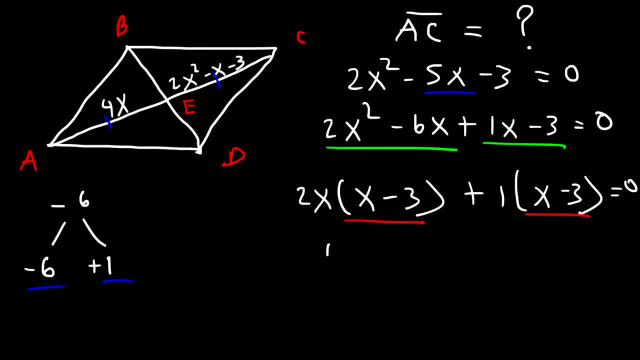 If these two are the same, that means you're on the right track. So we're going to factor out x minus 3, and then what goes inside the second parenthesis is what we see out here: 2x plus 1.. And so that's how you can factor this particular trinomial. 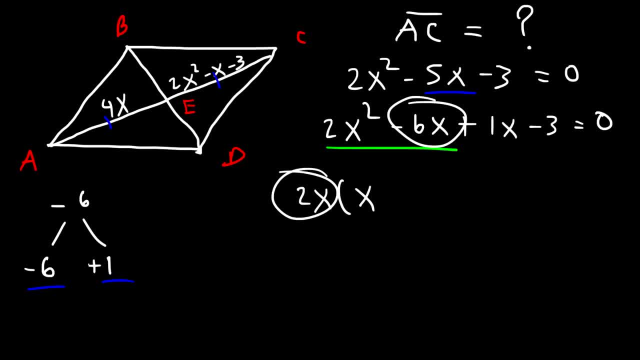 Is x Negative. 6x divided by 2x is negative 3.. Now, in the last two terms, factor out the GCF. If there is no GCF, factor out a 1, which means what's going to be on the inside is the same. 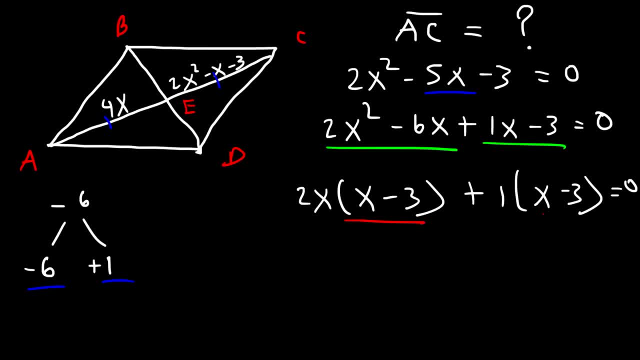 x minus 3.. If these two are the same, that means you're on the right track. So we're going to factor out x minus 3.. And then what goes inside the second parentheses is what we see out here: 2x plus 1.. 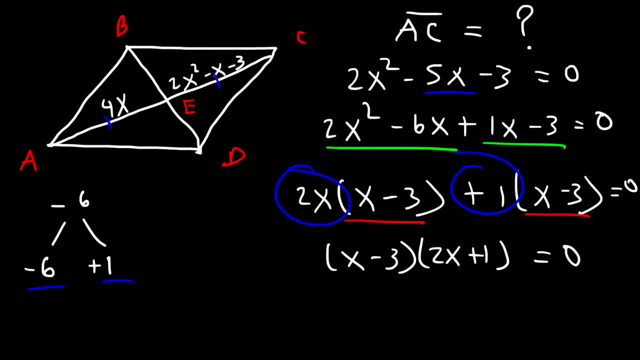 And so that's how you could factor this particular trinomial. Now, just like before, let's set each factor equal to 0. So for this one, let's add 3 to both sides, So we can see that one possible answer is that x is equal to 3.. 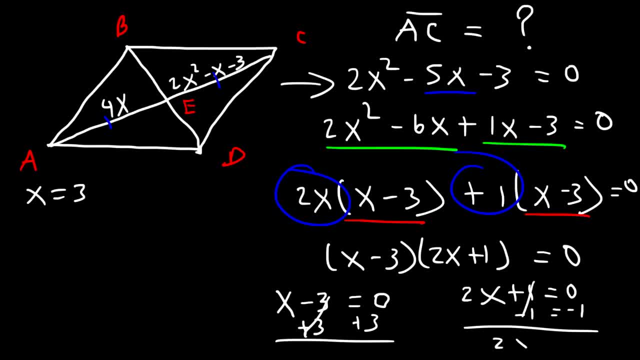 Now here let's subtract both sides by negative 1. So 2x is equal to negative 1. And then we'll have to divide both sides by 2.. So the other possible answer is that x is negative 1 half. 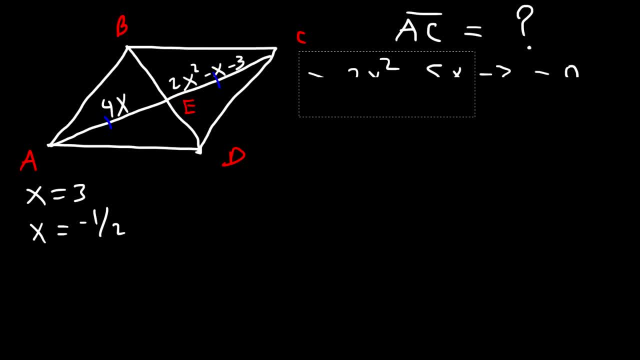 Now, which x value should we use? Can we use both of them, like the last problem, or just one of them? Now notice that if we plug in negative 1 half into 4x, it gives us a negative value And you can't have a negative length. so therefore this answer doesn't make sense. 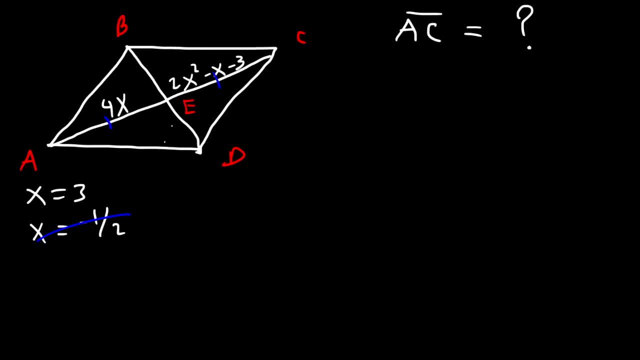 Now if the negative x value gave us a positive 4x value, or let's say, if that was 4x squared, then it would work. But you can't have a negative side length It just it is not practical. 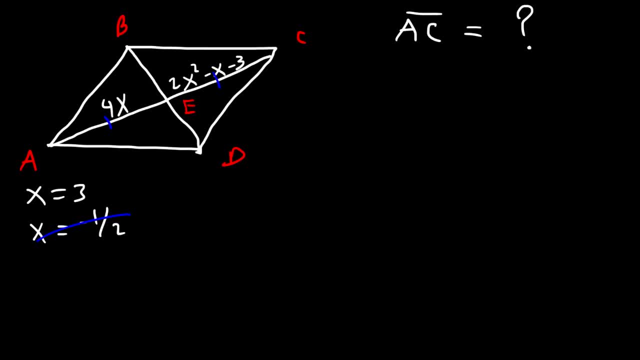 Like. what would that mean? So x has to equal 3 in this example. Now, ae is 4x, So it's 4 times 3, that's 12.. ec is 2x squared minus x minus 3, or 2 times 3 squared minus 3 minus 3.. 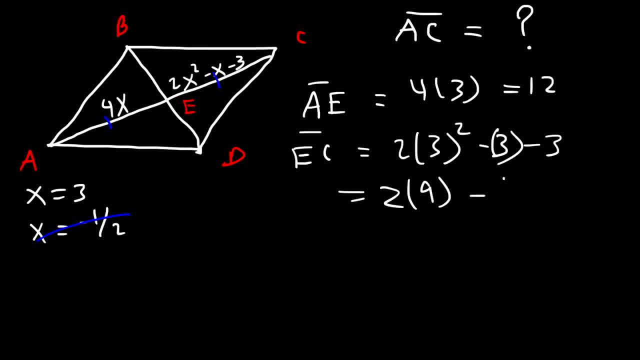 3 squared is 9, and negative 3 minus 3 is negative 6.. 2 times 9 is 18,. 18 minus 6 is 12.. So we can see that these two are indeed the same. Now, ac is the sum of ae. 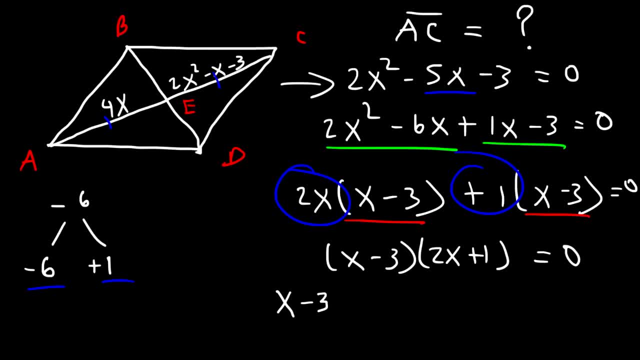 Now, just like before, let's set each factor equal to 0.. So for this one, let's add 3 to both sides, So we can see that one possible answer is that x is equal to 3.. Now here let's subtract both sides by negative 1.. 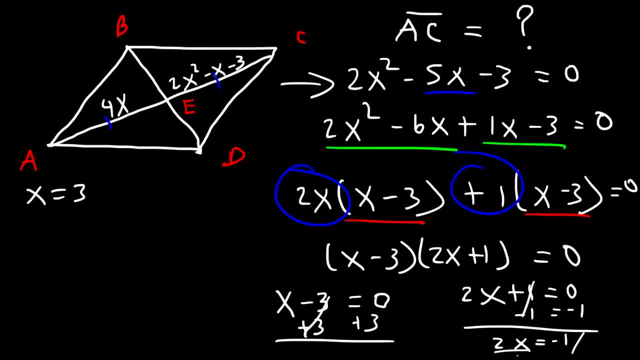 So 2x is equal to negative 1.. And then we'll have to divide both sides by 2.. So the other possible answer is that x is equal to 3. So we can subtract both sides by 2. that x is negative 1 half. now which x value should we use? can we use both them? 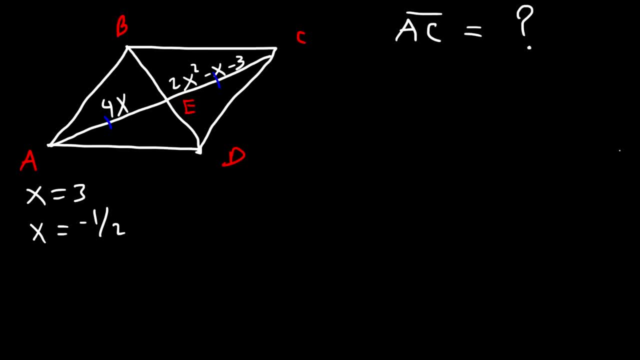 like the last problem, or just one of them. now notice that if we plug in negative 1 half into 4x, it gives us a negative value and you can't have a negative length. so therefore this answer doesn't make sense. now, if the negative x. 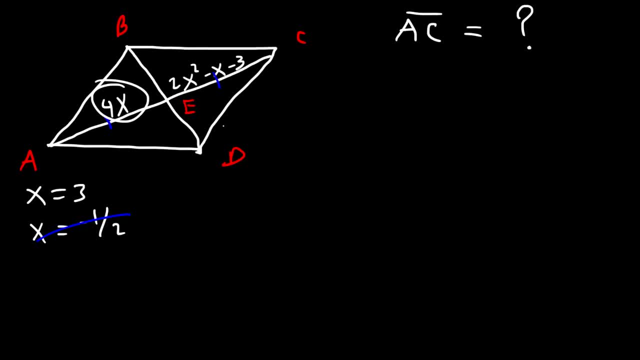 value gave us a positive 4x value. or let's say, if that was 4x squared, then it would work. but you can't have a negative side length it just it is not practical. like what would that mean? so X has to equal 3 in this example. now AE is 4x, so 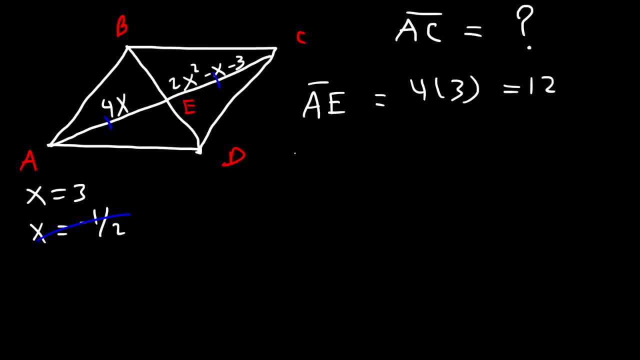 it's 4 times 3, that's 12. EC is 2x squared minus x minus 3, or 2 times 3 squared minus 3 minus 3. 3 squared is 9 and negative. 3 minus 3 is negative. 6 2 times 9 is 18. 18 minus 6 is 12. so we can see that these 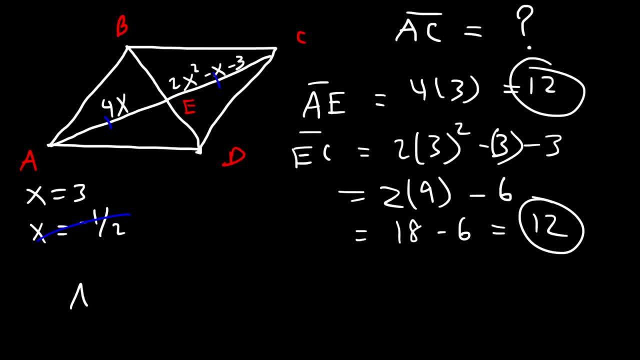 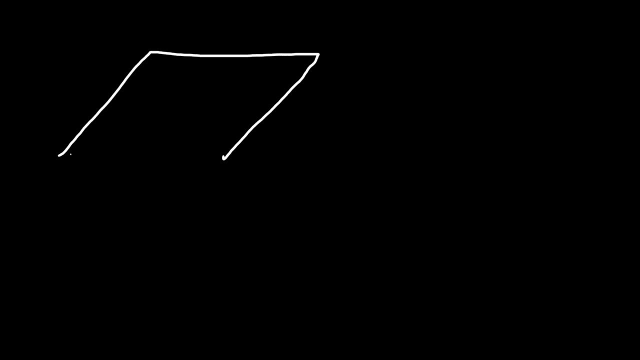 two are indeed the same. now, AC is the sum of AE and EC. so AE is 12, EC is 12. therefore, AC is 24, and this is the answer that we're looking for in this problem. here's another math problem for you, so we're going to use the same letters: ABC. 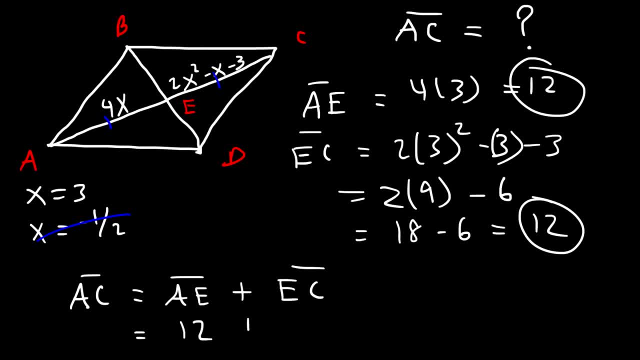 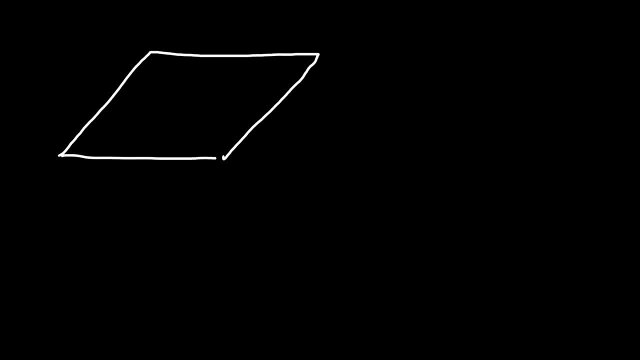 And ec. So ae is 12,, ec is 12,, therefore ac is 24.. And this is the answer that we're looking for in this problem. Here's another math problem for you. So we're going to use the same letters: a, b, c, d. 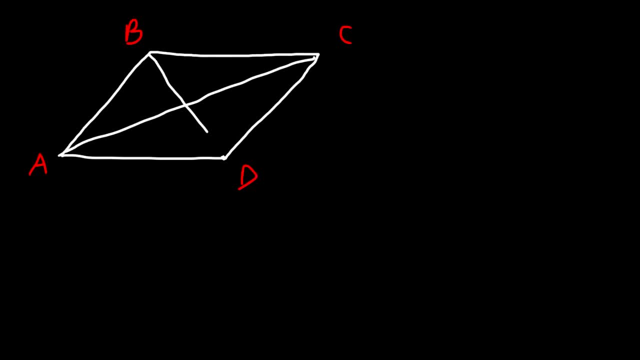 And once again we're going to have diagonals in this picture And this is e once again. So let's say that b e is 4x minus 6.. And b d, we're going to say it's 7x minus 8.. 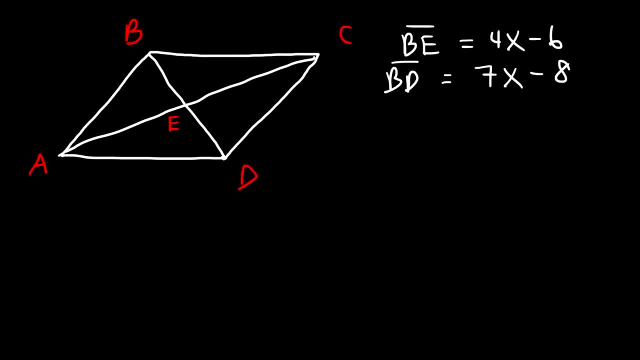 So, with this information, calculate the length of ed. Go ahead and work on it. So what's the relationship between b e and b d? Notice that b e is 1 half of b d. So let's say if b e was 7, that means ed would be 7,. 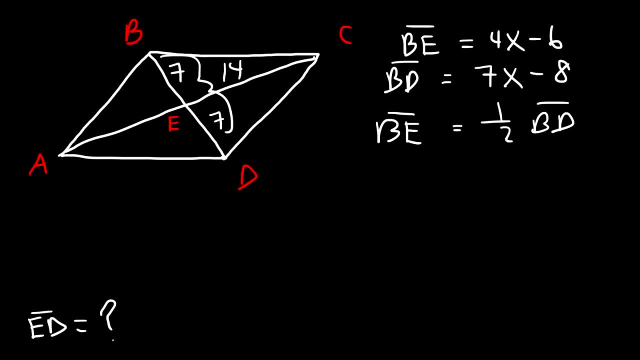 but b d would be 14.. 7 is 1 half of 14, for example. So b e is 4x minus 6.. b d is 7x minus 8.. What I'm going to do is I'm going to multiply both sides by 2. 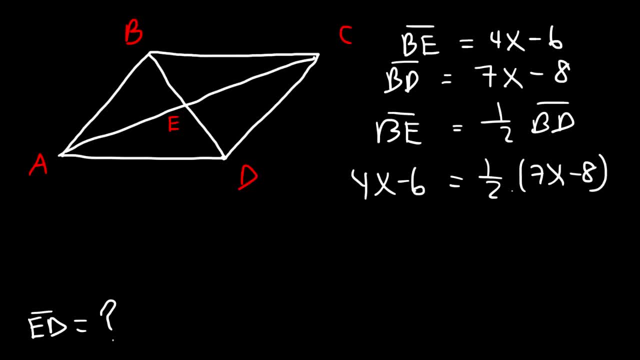 because if I distribute the 1 half, I'm going to have 7 over 2.. And I don't want any fractions. So let's multiply this side by 2 and the left side by 2.. So 1 half times 2 is 1.. 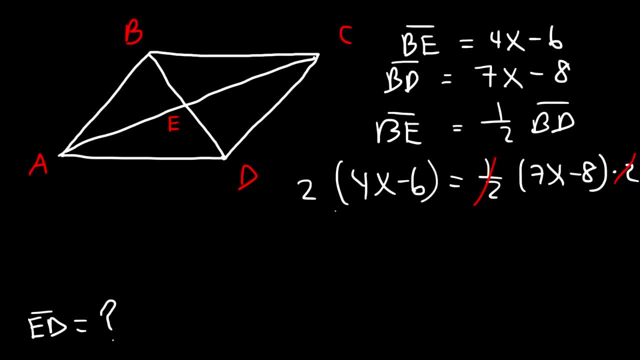 Now on the left side, I need to distribute the 2 to 4x minus 6.. So 2 times 4x is 8x And 2 times negative 6 is negative 12.. On the right side, because I cancelled the fraction: 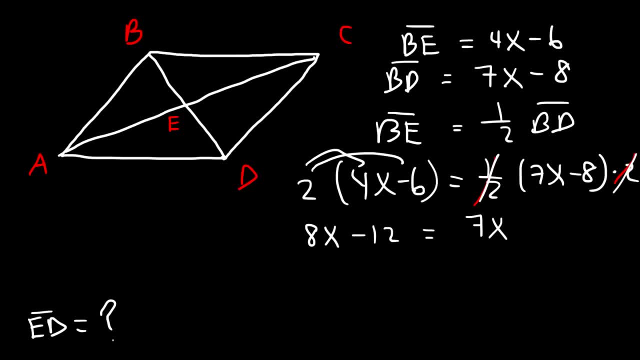 I no longer need a parenthesis, so I can simply write 7x minus 8.. Now let's subtract both sides by 7x And let's add 12 to both sides, So these two will cancel. 8x minus 7x is 1x, which is simply x. 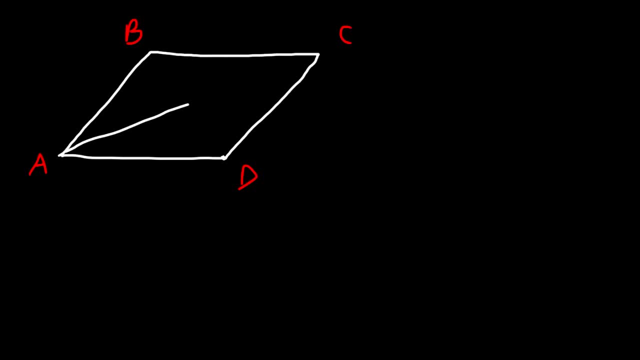 D and once again we're going to have diagonals in this picture and this is e, once again. so let's say that be is 4x minus 6 and BD. we're going to say it's 7x minus 8. so with this, 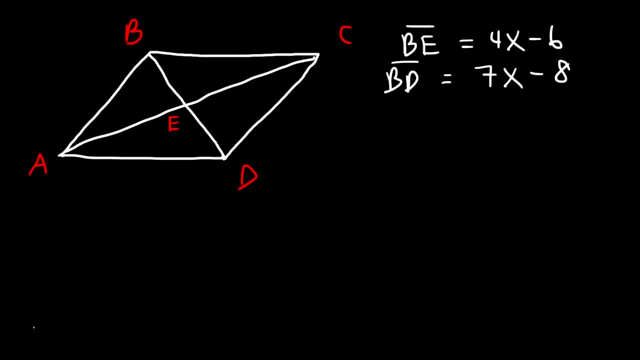 information, calculate the length of ed, go ahead and work on it. so what's the relationship between the e and BD? notice that be is one half of BD. so let's say, if be was 7, that means ed would be 7, but BD would be 14. 7 is one half of 14. for 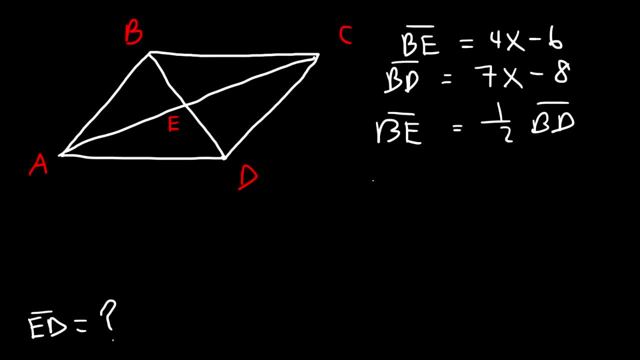 example. so be is 4x minus 6. BD is 7x minus 8. what I'm going to do is I'm going to multiply both sides by 2, because if I distribute the one half, I'm going to have 7 over 2. 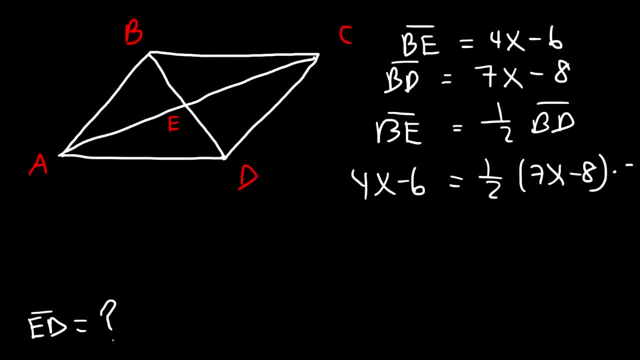 and I don't want any fractions, so let's multiply this side by 2 and the left side by 2. so one half times 2 is 1. now on the left side, I need to distribute the 2 to 4x minus 6. 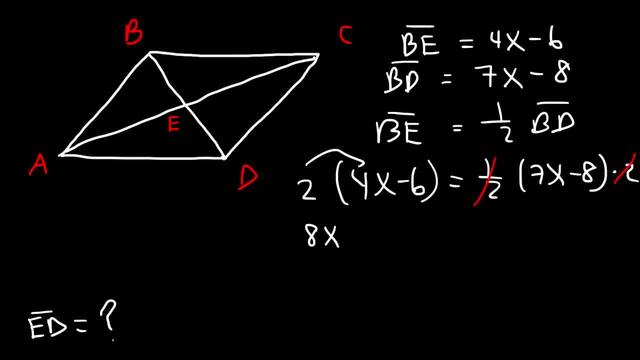 so 2 times 4x is 8 x and 2 times negative 6 is negative 12. on the right side. because I cancel the fraction, I no longer need a parentheses, so I can simply write 7x minus 8. now let's subtract both sides by 7x and let's add 12 to both sides, so these two 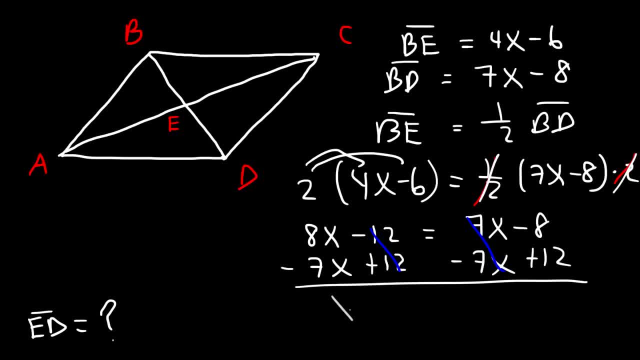 will cancel. 8x minus 7x is 1x, which is simply x, and negative. 8 plus 12 is 4, so now we have the value of x. x is equal to 4, so now we can calculate BE. so that's 4x minus 6 or 4 times 4 minus 6. 4 times 4 is 16. 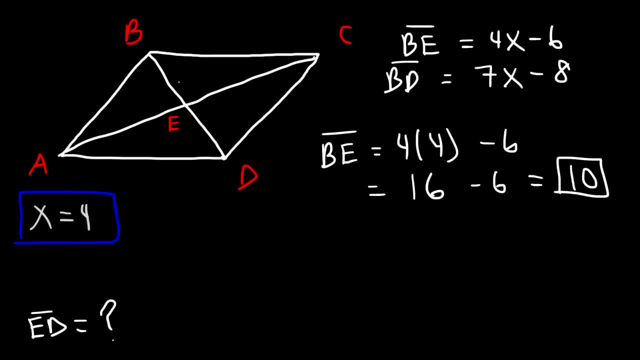 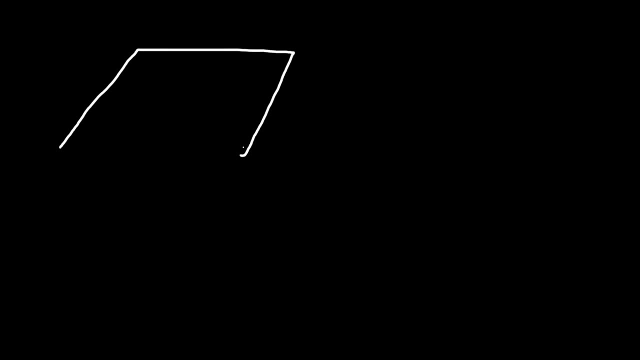 and 16 minus 6 is 10, so BE is 10, which means ED is also 10, and so that's the answer: ED is 10 units long. now let's consider another problem. so this one is going to be a little bit different than the other ones. 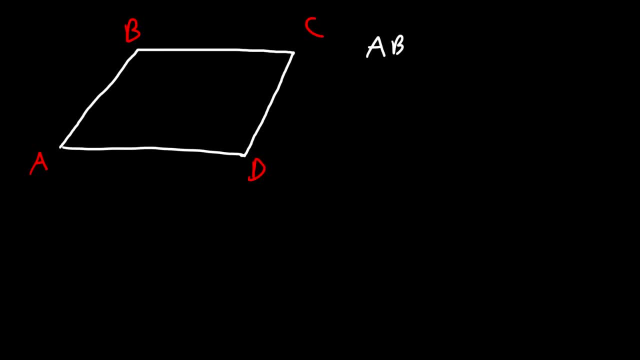 so let's say that AB is equal to 3x plus 4, and let's say BC is equal to 5y plus 3, and CD is equal to 7x minus 12, and also AD is 2y plus 12.. So with this information, calculate the. 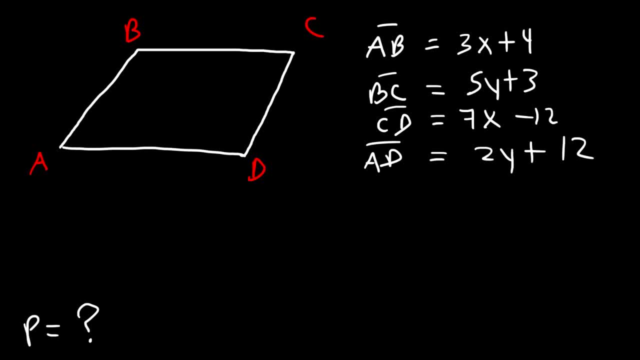 perimeter of the parallelogram. Go ahead and try it. So keep in mind: opposite sides are congruent Now. AB is 3x plus 4 and BC is 5y plus 3.. That doesn't look like a y, so let's fix that. And CD is 7x minus 12. 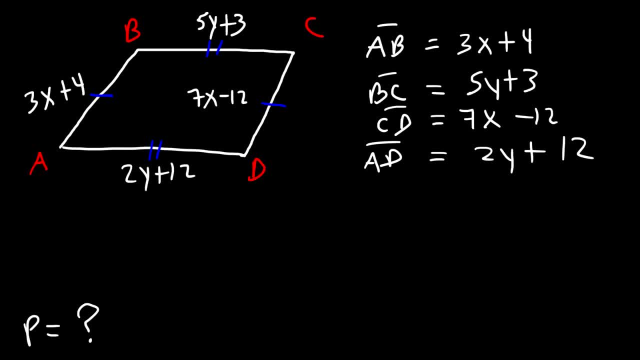 AD is 2Y plus 12.. So since opposite sides are congruent, we know that AB is congruent or equals CD. So AB is 3X plus 4. We can set that equal to 7X minus 12.. 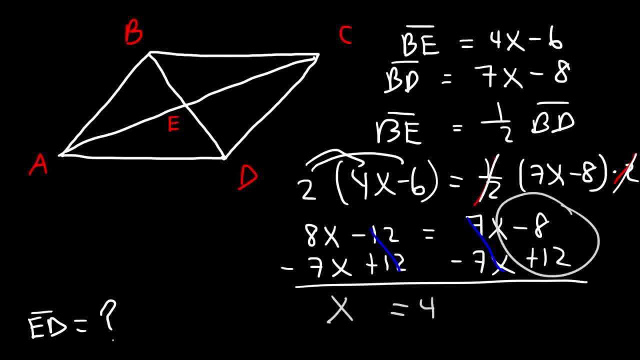 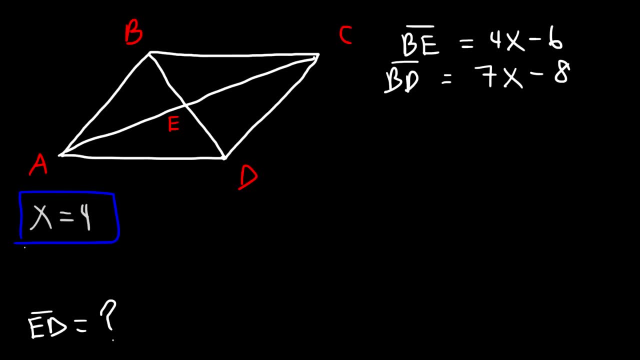 And negative 8 plus 12 is 4.. So now we have the value of x. x is equal to 4.. So now we can calculate b, e. So that's 4x minus 6, or 4 times 4 minus 6.. 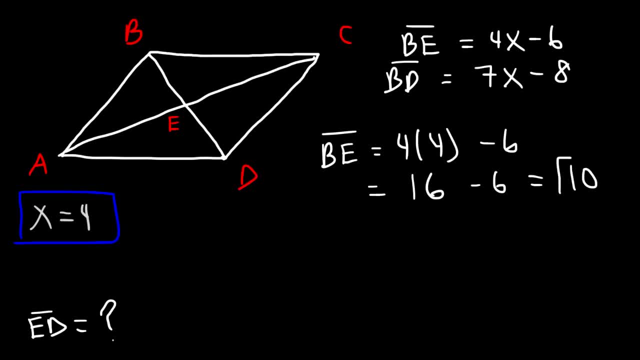 4 times 4 is 16. And 16 minus 6 is 10.. So b? e is 10,, which means e d is also 10.. And so that's the answer: e d is 10 units long. 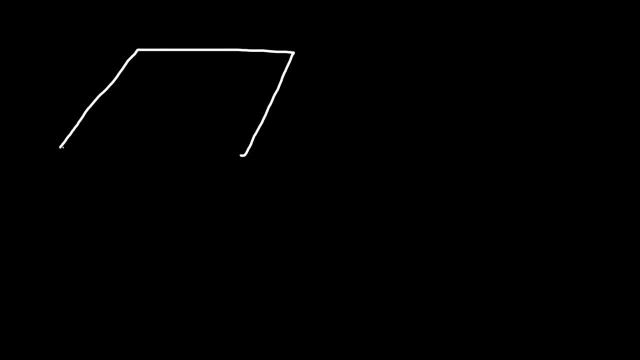 Now let's consider another problem. So this one is going to be a little bit different than the other ones. So let's say that a- b is equal to 3x plus 4.. And let's say b- c is equal to 5y plus 3.. 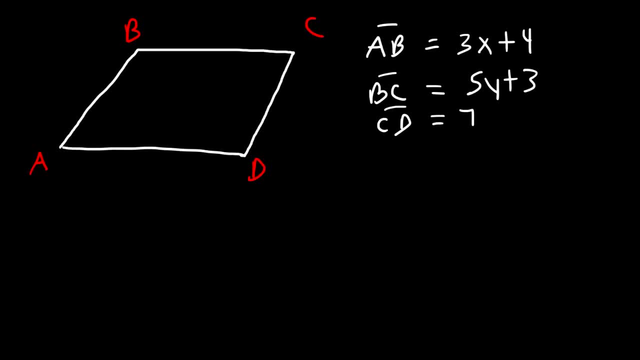 And c, d is equal to 7x minus 12.. And also a- d is 2y plus 12.. So with this information, calculate the perimeter of the parallelogram. Go ahead and try it. So keep in mind. 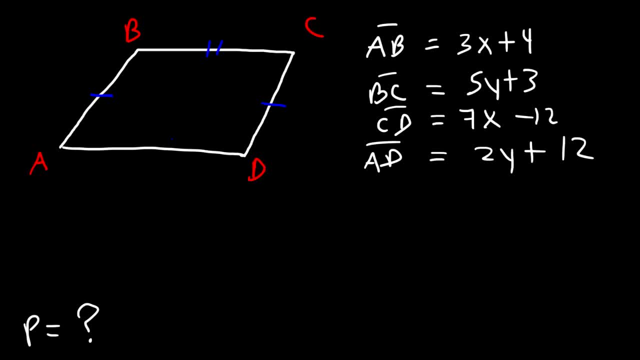 opposite sides are congruent Now: a- b is 3x plus 4. And b- c is 5y plus 3.. Okay, that doesn't look like a- y, So let's fix that. And c- d is 7x plus 12.. 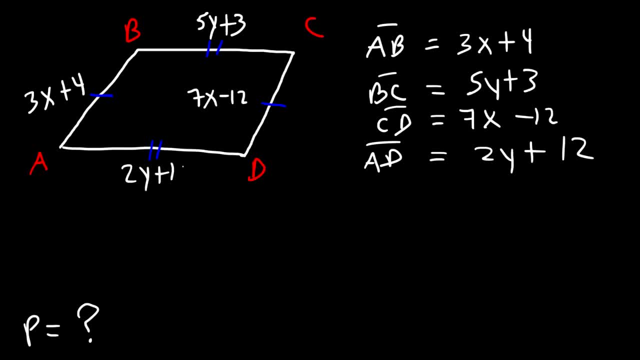 So we get 7x minus 12.. a- d is 2y plus 12.. So since opposite sides are congruent, we know that a- b is congruent or equals c- d. So a- b is 3x plus 4.. 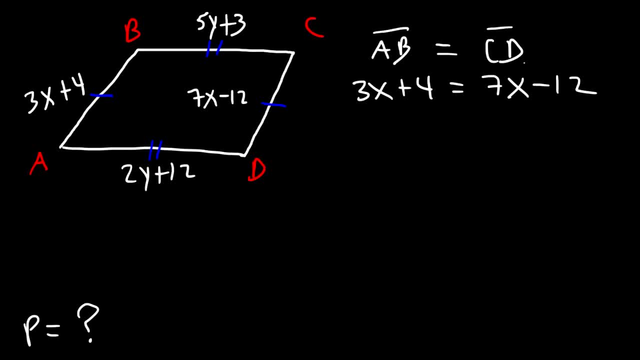 We can set that equal to 7x minus 12.. So let's subtract both sides by 3x And let's add 12 to both sides And we have: 4 plus 12 is 16.. And 7x minus 3x is 4x. 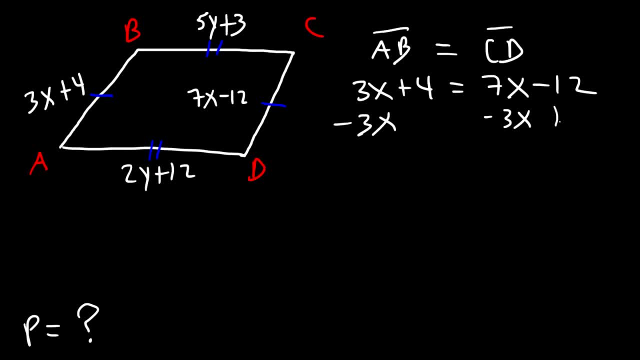 So let's subtract both sides by 3X And let's add 12 to both sides. 4 plus 12 is 16.. And 7X minus 3X is 4X. So if we divide both sides by 4, 16 divided by 4 is 4.. 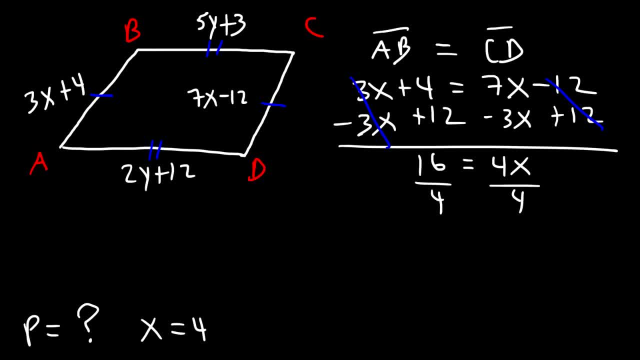 So X is equal to 4.. Now, if X is equal to 4, we can calculate the measure of side AB. So AB is 3X plus 4.. So that's going to be 3 times 4 plus 4.. 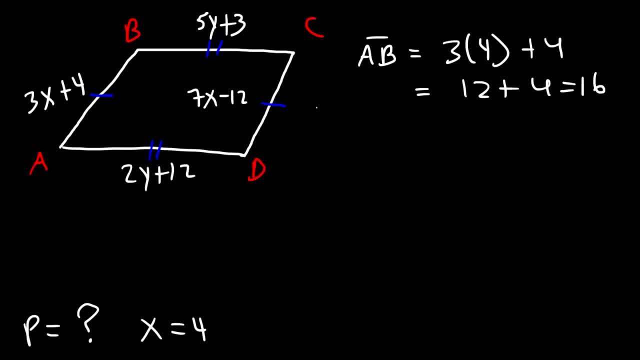 And so this is 12 plus 4, which is 16.. So CD and AB: they're both equal to 16, since they're congruent to each other. Now we could also set BC equal to AD, because they have the same length. 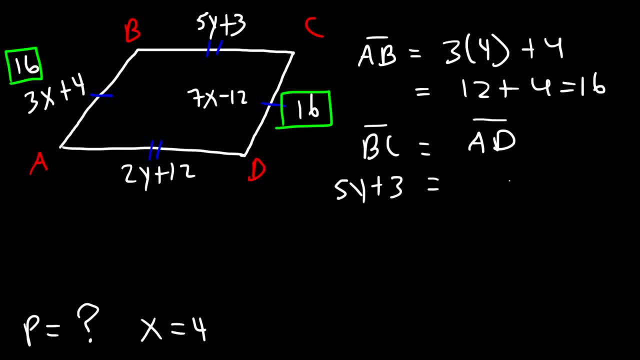 Now BC is 5Y plus 3. AD is 2Y plus 12. So let's subtract both sides by 2Y and by 3.. 5Y minus 2Y is 3X. 12 minus 3 is 9.. 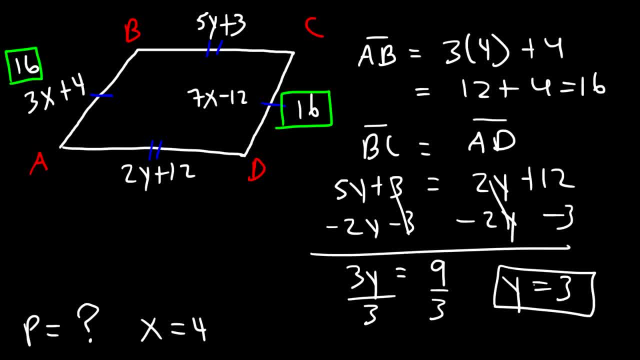 And 9 divided by 3 is 3.. So now we can find the measure of BC. So it's 5Y plus 3. So that's 5 times 3 plus 3.. 5 times 3 is 15.. 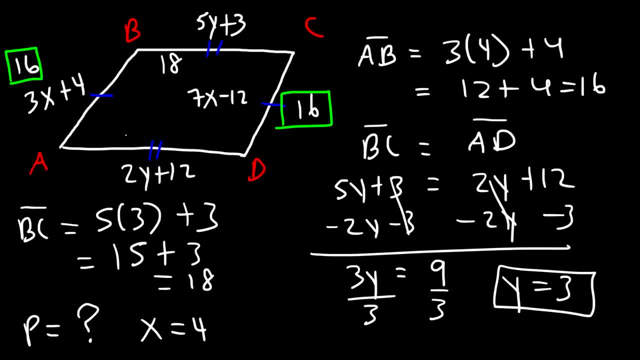 15 plus 3 is 18.. So BC and AD, they both equal 18.. So now we can calculate the perimeter. The perimeter is going to be 2 times 16, because we have two of them plus 2 times 18.. 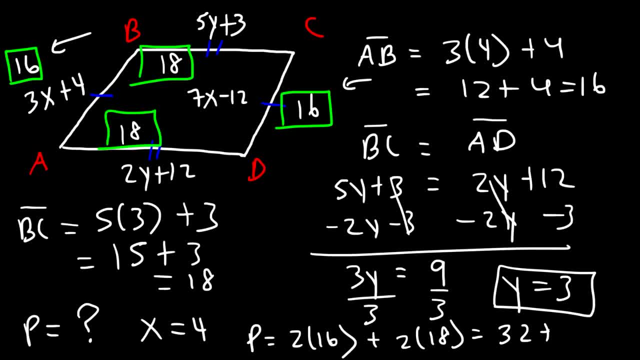 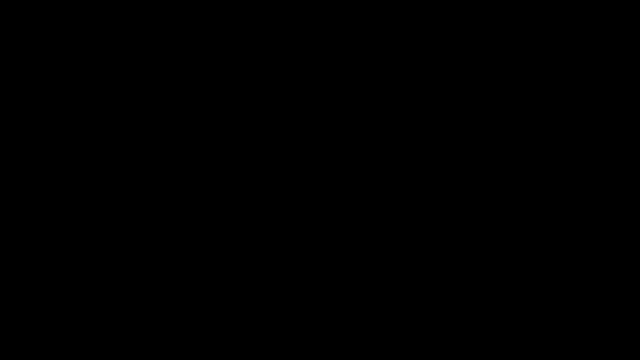 So 2 times 16 is 32.. 2 times 18 is 36.. 32 plus 36 is 68.. So that's the perimeter of this particular quadrilateral. So we have 2 times 1.. And 2 times 6 is the perimeter of that particular quadrilateral. 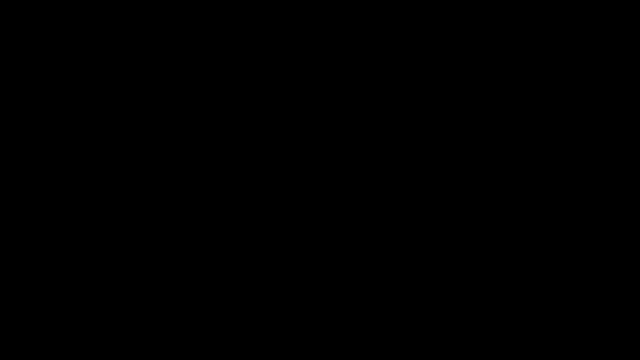 So the perimeter of that quadrilateral is 18.. So from this point we got the perimeter, So don't forget to connect the two terminals. And then we start to see the perimeter of this quadrilateral, And then you can now see that we have 1.. And then we are going to see that we have a bit of a fence between this two. So we got the perimeter of the quadrilateral and this square, And that's because we have 2 times 6.. So we have to be careful. We need to be careful.